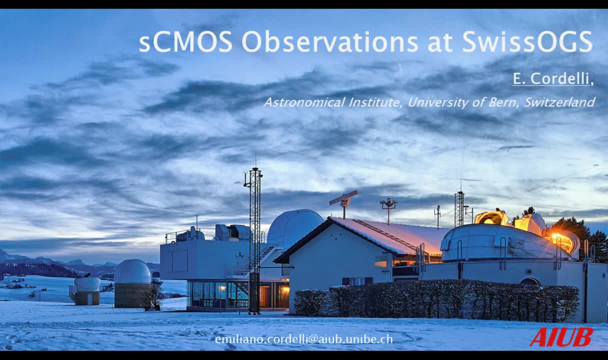 and we encourage you to participate by submitting as many questions as you want at any time you want during the presentation. To do so, simply type them into the Ask a Question box and click Send. We will answer as many questions as we have time for at the end of the presentation. 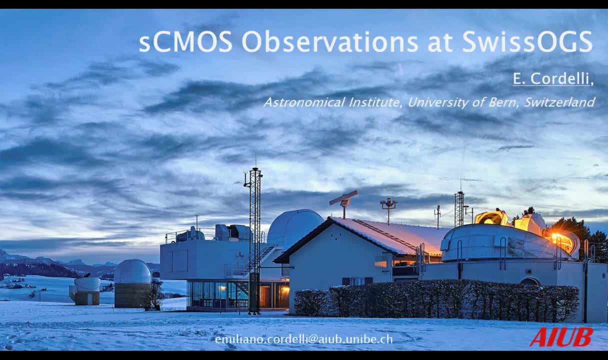 If you have any trouble seeing or hearing the presentation, just use that Ask a Question box to let us know you're experiencing a problem. Today's webinar is educational and thus offers continuing education credits. Just click on that Continuing Education Credits tab at the top of. 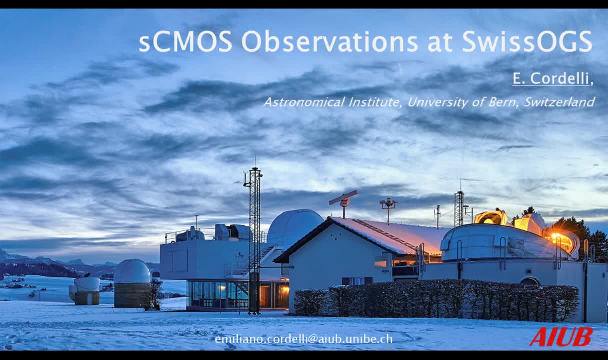 your screen and follow the process to obtain your credits. I would now like to introduce our first speaker, Dr Emiliano Cordelli. Dr Cordelli is a researcher at the Astronomical Institute of the University of Bern and currently in charge of research and. 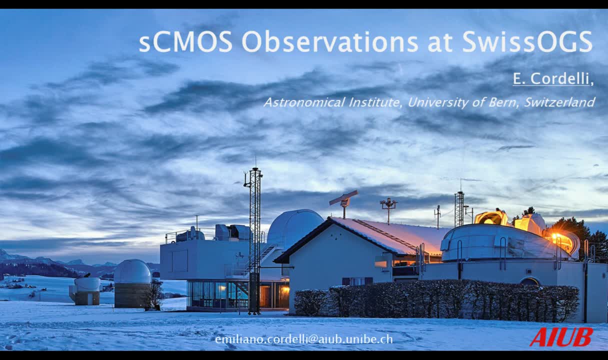 development at the Swiss Optical Ground Station and Geodynamics Observatory Dimmerwald, Swiss OGS. His areas of expertise include orbital and attitude dynamics of artificial objects, covering also the orbit and attitude determination of space debris. He has observational and analysis experience of satellite laser ranging, astrometric and photometric measurements. 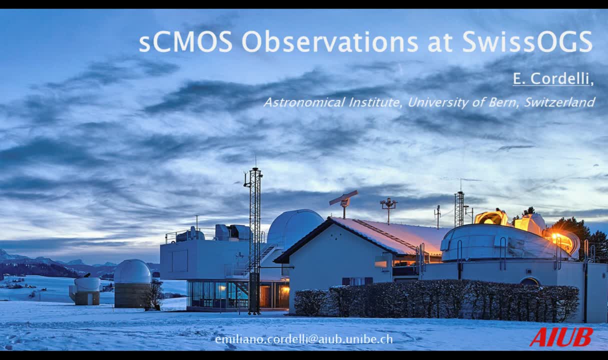 For a complete biography on Emiliano, please visit the Biography tab at the top of your screen. Emiliano, you may now begin your presentation. Thanks, Christe. Hello everybody. Today I would like to talk to you about some CMOS. 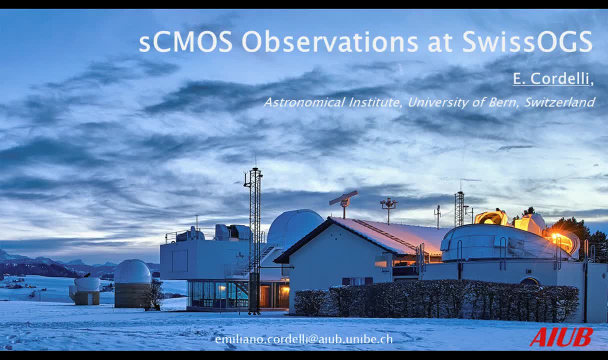 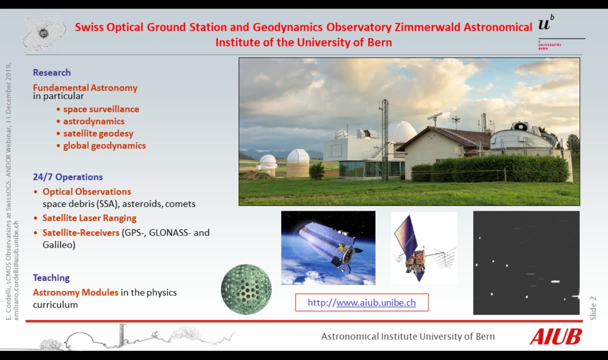 observations that we performed here at the Swiss Optical Ground Station Geodynamics Observatory Dimmerwald. So just a small presentation first. The Swiss Optical Ground Station Geodynamics Observatory in Dimmerwald belongs to the Astronomy Institute of the University of Bern. Here we perform. 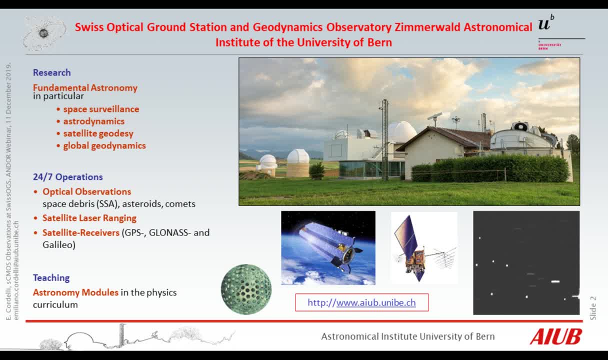 research activity focusing on the space debris, on the space surveillance, astrodynamics, satellite geodesy and global geodynamics. In order to support these research activities, the Swiss OGS is performing 24-7.. Our telescope during the night observes especially space debris, asteroids, comets and supernovae. 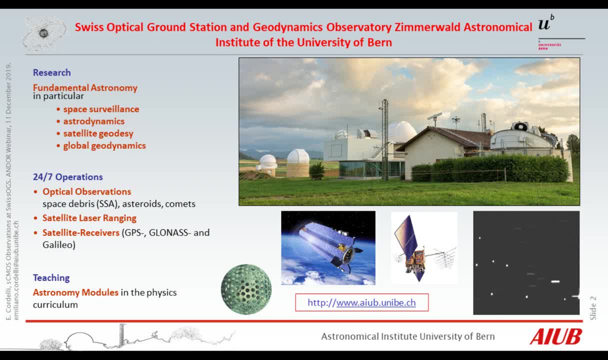 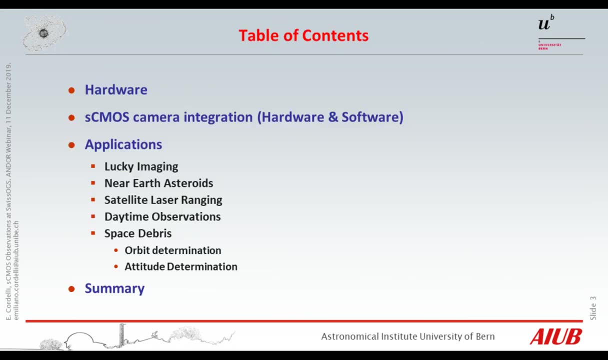 while during daytime and nighttime we have a satellite laser ranging system and a GPS receiver or GNSS receiver working 24 hours per day. Of course, being part of the university, we have also some teaching module in astronomy. A short outline of this talk. I will briefly talk at the beginning about the spé cloves. 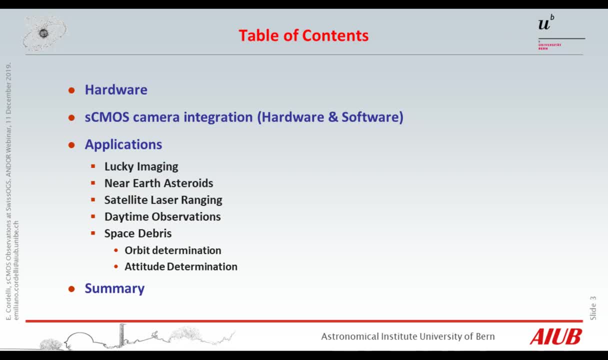 where the camera, the CMOS camera, is integrated and which software we needed to develop in Office 2 to do some particular observation, and then I will talk about the kind of observation that you are performing. So we do some- probably images, some observation about us online. and some trouble with computer certifications and softwares. In closing, we hope to be able to support you on your research. where did you offer things that you would want to use about your laboratory? the? the Port of sera, Theων Islandkar range harbour area for penguins flying 500m. 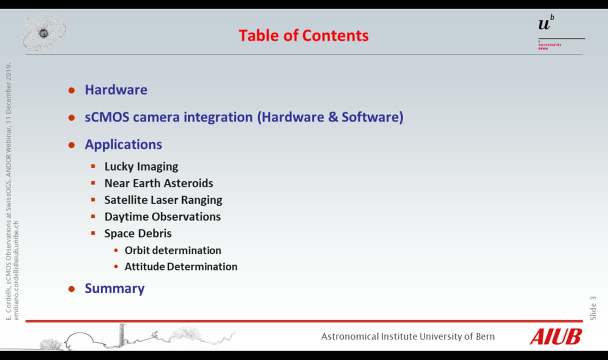 The camera is also used as a tracking camera in parallel to the satellite laser ranging activities. Then we were able recently to extend our camera observation also to daytime operation. and finally, what we can get in terms of space debris and how we can, how this measurement. 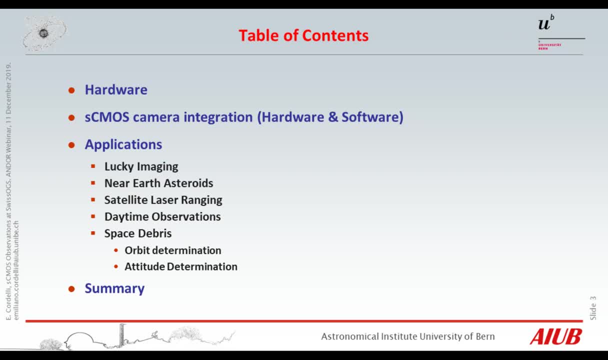 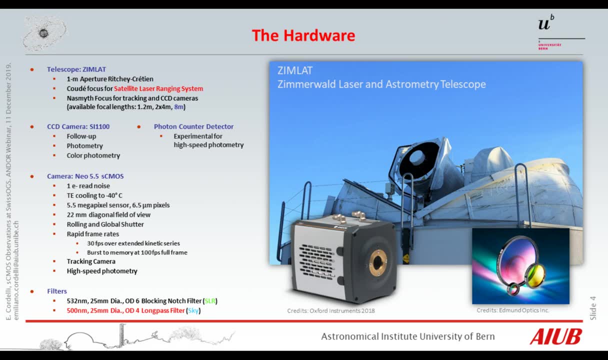 can be useful for orbit and attitude determination. Okay, starting from the hardware, So all the observations that we will see later on are acquired with the Timurvan Laser and Astronomy and Astrometry Telescope. This is one meter class telescope. It's pretty versatile. 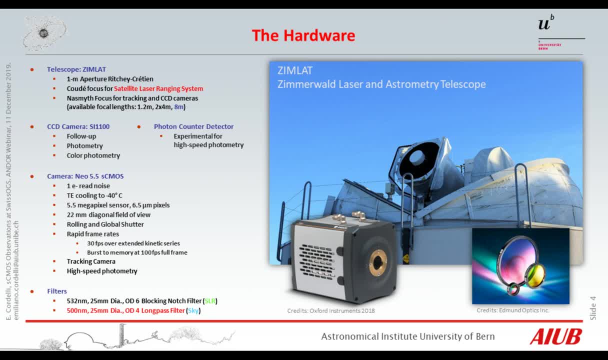 We have different experiments ongoing on this telescope. We have, as an example, one coup de passe for the satellite laser ranging system. Then we have in the NASMIT platform we have four focal stations with different focal lengths. In one there is a CCD camera. 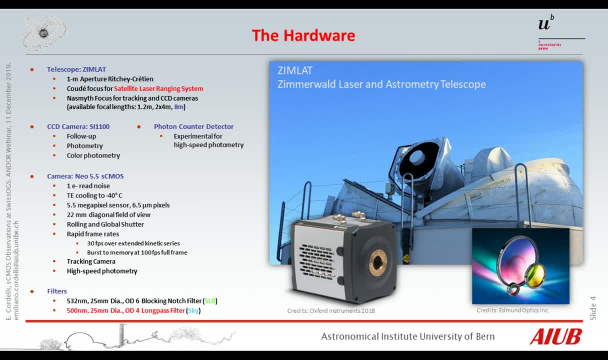 In one. there is a photon counter detector that is just for experimental use and we and is under testing at the moment. And then today we will talk about mainly the operation that we perform on the CMOS camera. Since the CMOS camera was created, we have been using it for a long time. 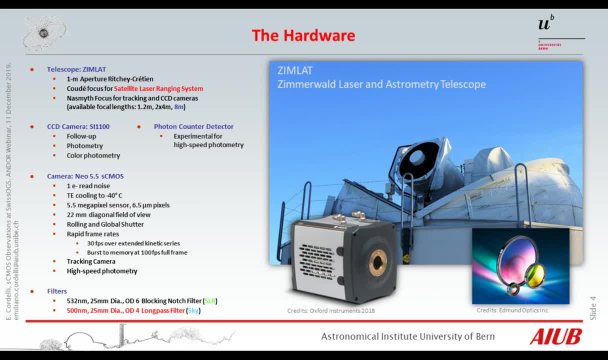 Since the CMOS camera was created, we have been using it for a long time. Since the CMOS camera is running in parallel to the laser observation, we needed to add the filter to block the laser light. The laser light reaches the sensor. because we don't want to damage the camera. 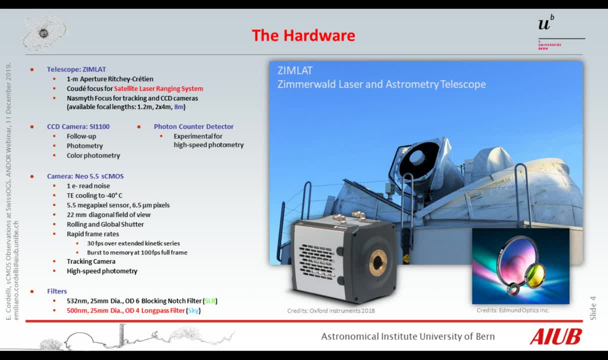 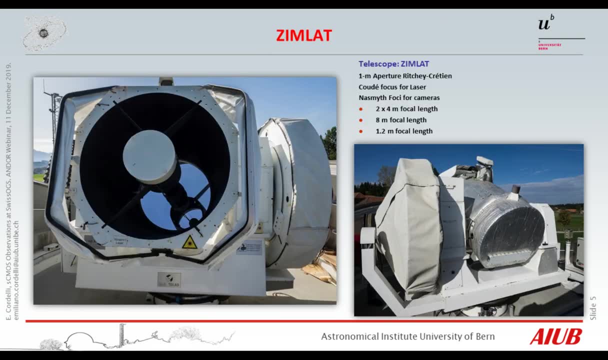 And then, since we extended also the observation during daytime, we added also a sky filter to cut out the light of the sky, as we will see later. So once again, this is a CMOS camera. This is our telescope, some particular in front, from the back, and we have the NASMIT. 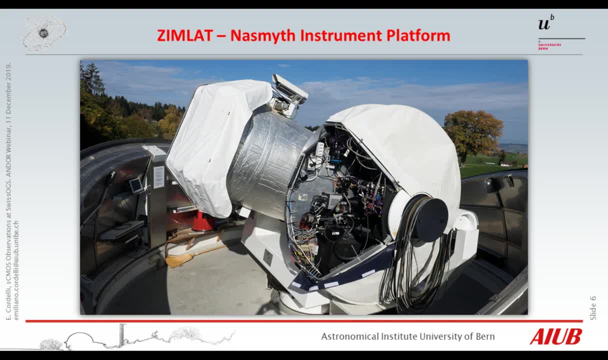 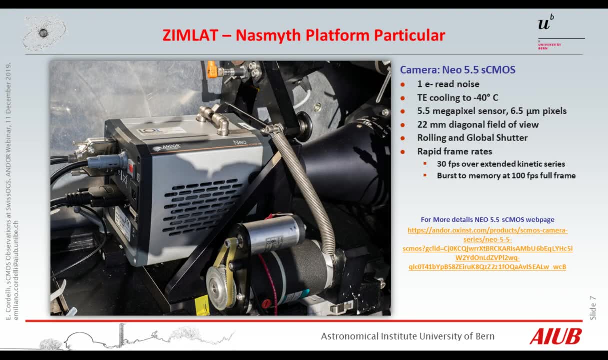 platform. Why the NASMIT platform is interesting for us? Because, as we can see, here there is the camera installed and just the particular. here you see how the camera fit and on the right of the picture you have the focal reducer. We have the focal reducer. 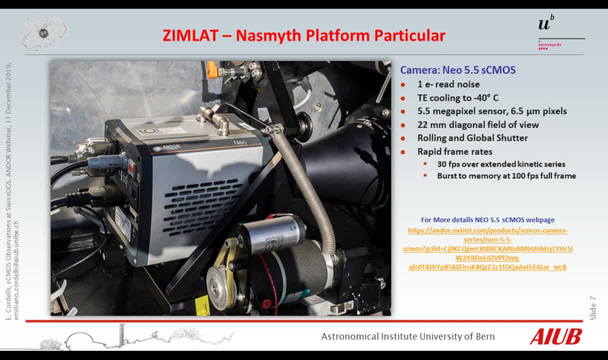 For more information, please visit our website. Thank you For detailed details about this camera. I will leave the link to go to the Andor website. What is interesting of just small information? the 22mm diagonal field of view of the camera. 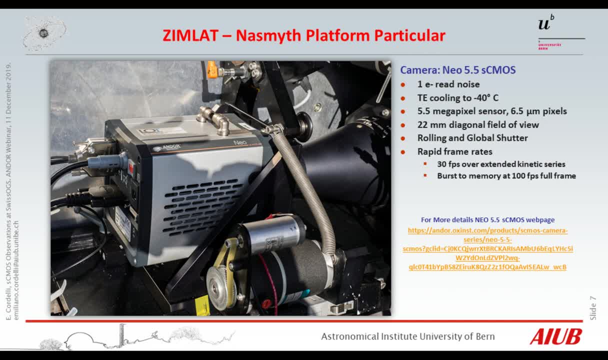 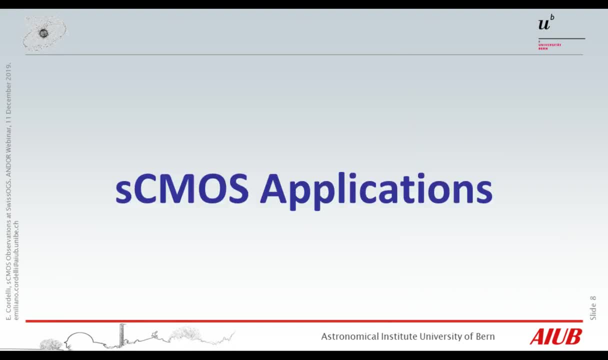 allow, on the focal length, that we are using the 8 m focal length, a field of view of 6 by 7 arc-minutes. It is important for the our application. Thank you for the application that we are going to see now. so, starting with the application we know being 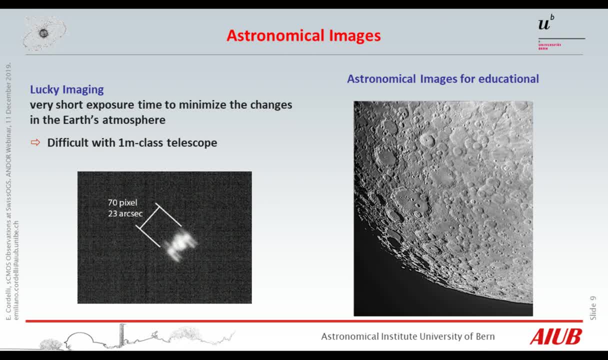 research institute, part of the university, we are also performing some educational observations. so in the right part, in the right side of the slide, we see and the results of a series of images acquired for the moon. it seemed very nice to see, for students at least. it's very nice to see the 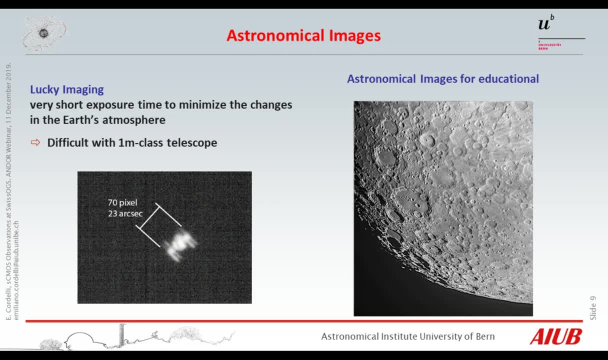 details the on the surface of the moon like craters, and actually it's easy, from a picture, measure the dimension of the craters and with some math more we can measure also the height of the mountains and of the crater, knowing the position of the sun and the position and the 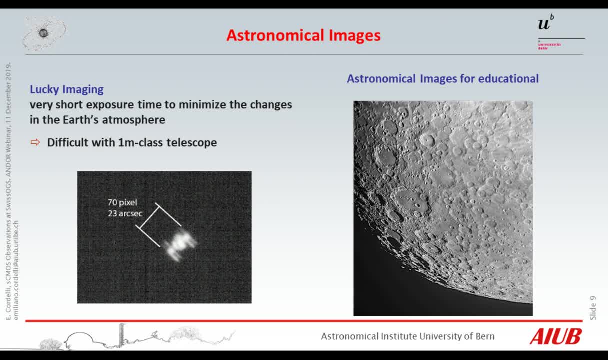 amount of the shadow that we see. then some funny tests, where we performed some funny tests with the lucky imaging. actually, we assume that the, the atmosphere is made by her lenses and, if you are lucky enough, one of these lengths will be on top of your telescope and will. 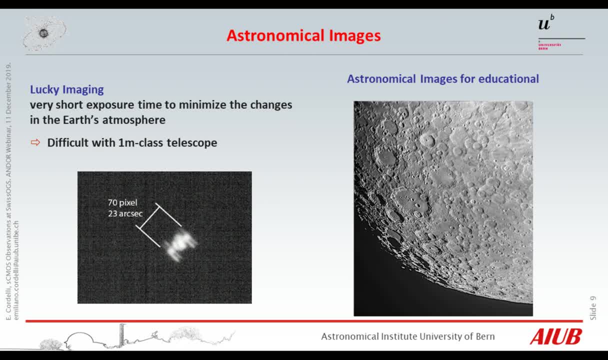 compensate the effect of your seeing, delivering so so very sharp images. so this is the problem is that for one meter telescope to have one meter, her lens is a bit more rare, so you don't have a perfectly sharp image, but nevertheless, here is interesting to see on the left picture, the, an image of the 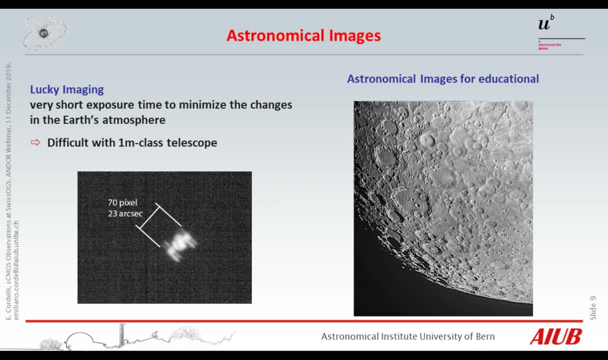 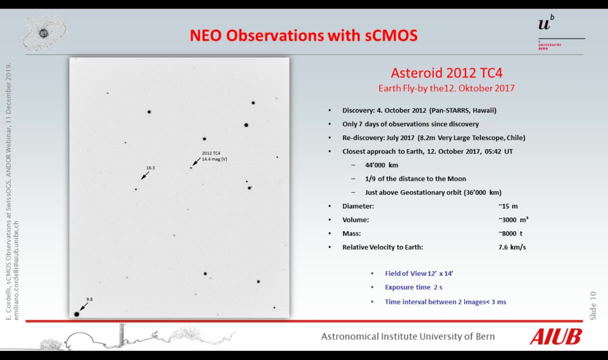 international space station from which you can distinguish- one can distinguish between the two, which is quite easily the body of the of the space station and the solar panels. okay, let's move for more, let's say scientific results. so this is a an example of the picture taken with the 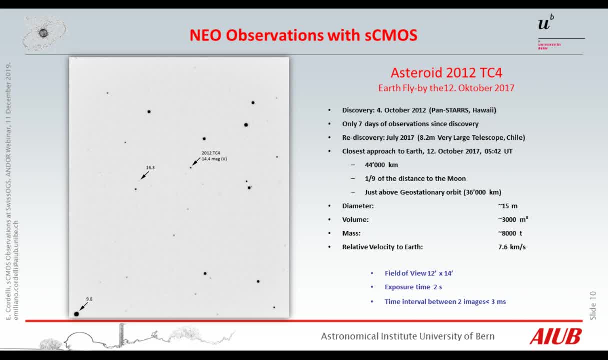 cmos camera when it was in the four meter focal length- the effective field of view, in fact, is 12 by 14 half minutes- and we perform an observation campaign of uh, the asteroid, the 2012 tc4, during its fly by around the earth. actually, this satellite- 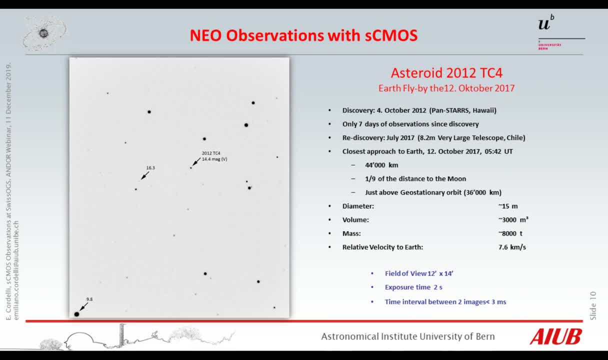 this picture was observed the night of the 11th of october and the satellite was- uh sorry, not satellite- the. this asteroid was passing at a distance of 44 000 kilometers from the earth. in terms of astronomical distances, this is pretty close, actually, and it just it was just 8 000 kilometers above the geostationary ring. 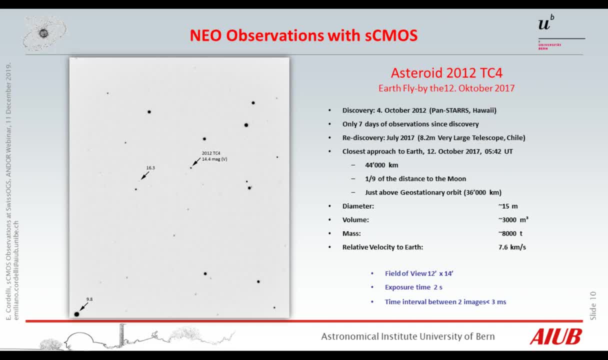 that is one of the most crowded space region that we use for human activities like television and remote sensing, a meteor observation. so what we can see? in the center of the image we see the asteroid, and then we have also the limit, let's say one of the 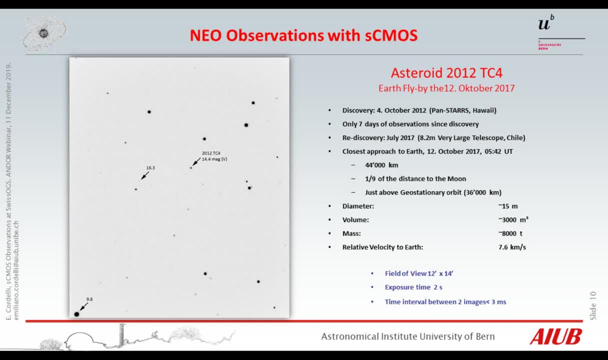 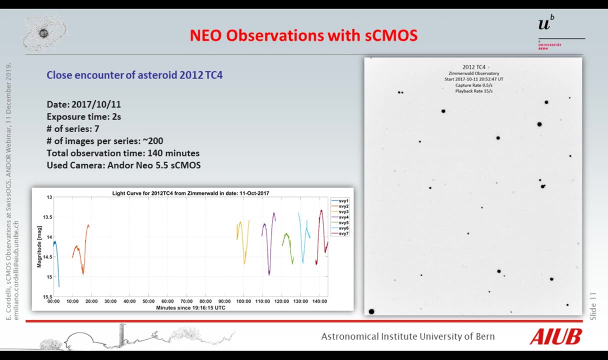 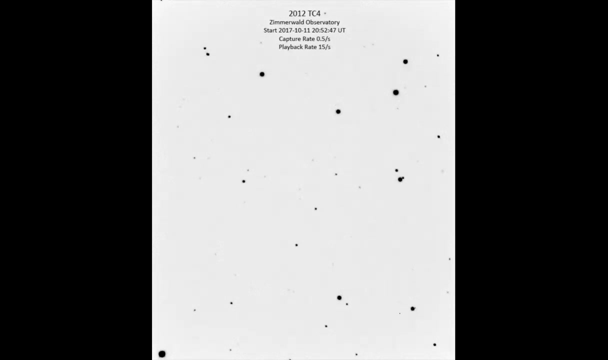 faint. we highlighted also one of the faintest stars that we could get with using this camera and only two seconds of exposure. so, um, but okay, this is just a picture. now i will show you a video about these, uh, these asteroids. so let's see how it looks from the analysis of this video. 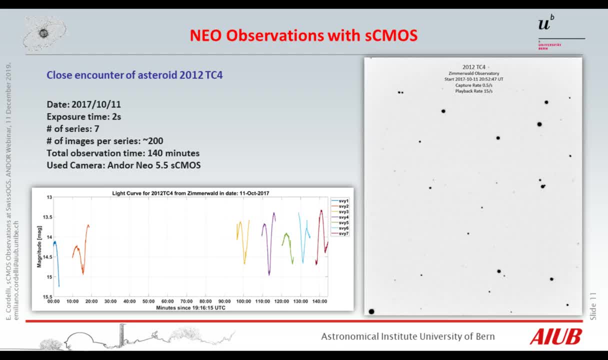 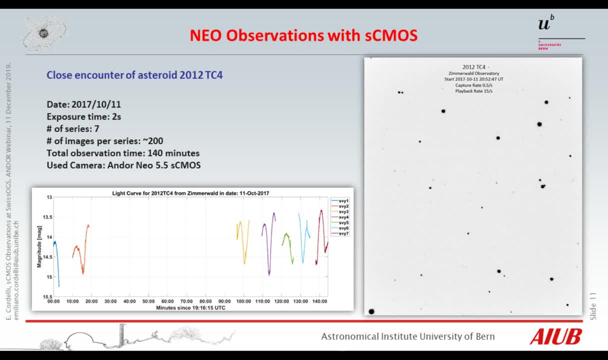 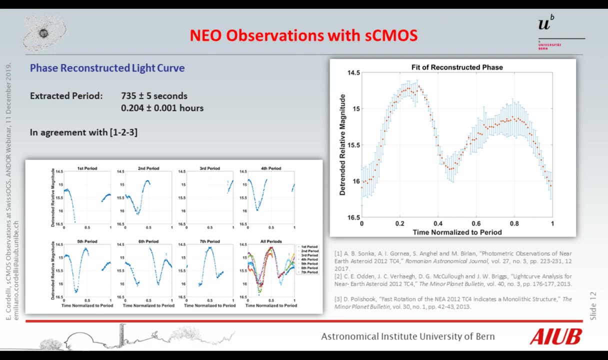 if we analyze the brightness variation of the light reflected by the asteroid over this image series, we get these segmented light curves. nevertheless, this segmented light curves allowed us to perform a phase reconstruction um of the phase reconstruction procedure that allowed to extract the phase diagram of the of the object that we can see on the right. 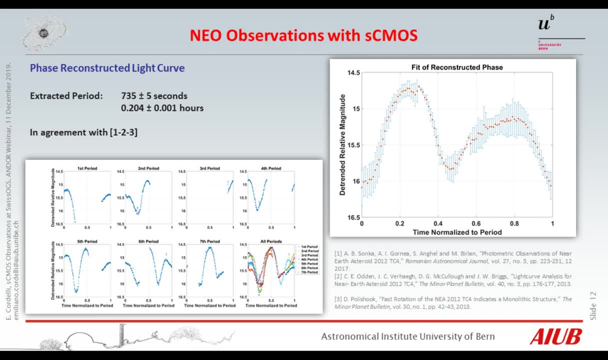 and once we are able to get a sharp phase diagram, we are also able to extract the rotation period of this asteroid. This is very interesting because, knowing the phase diagram, we can all the astronomers were inferring the shape of the asteroid, while we could extract also this rotation period. that was. 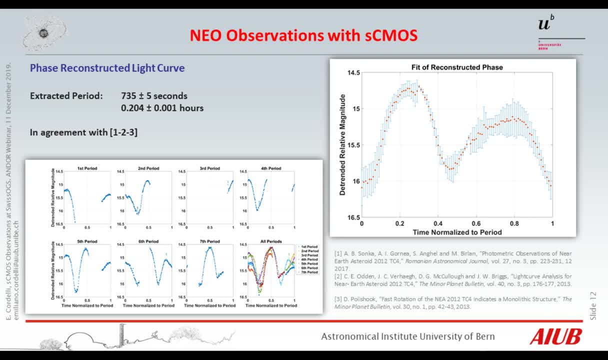 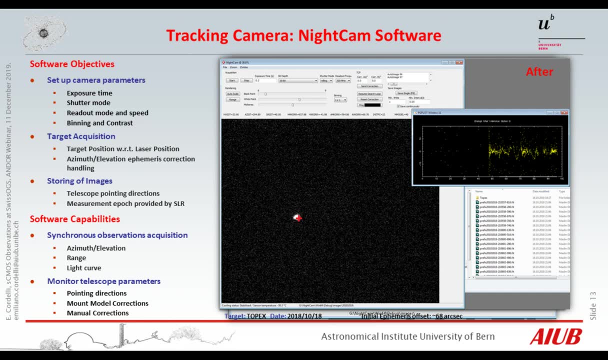 confirmed also by the results found in the literature. More extensive work on this CMOS camera was performed because we wanted to use the camera to support the satellite laser ranging observation. Actually, when performing a satellite laser ranging, we know already where the object is. and we know already where the object is. 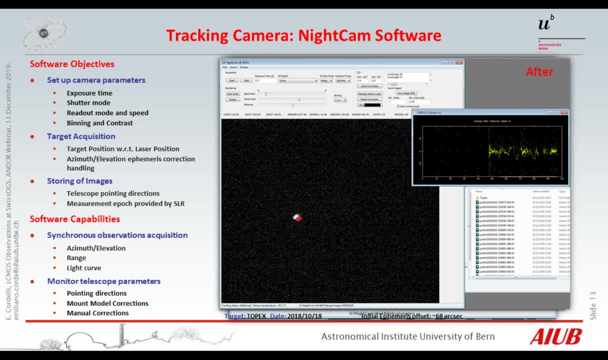 that we want to track is. This is usually a geodetic satellite whose orbits are really precise, but nevertheless some DFM rays are not accurate or not very accurate, or at least not always so. the idea was to use, to employ this camera to have a stream video. 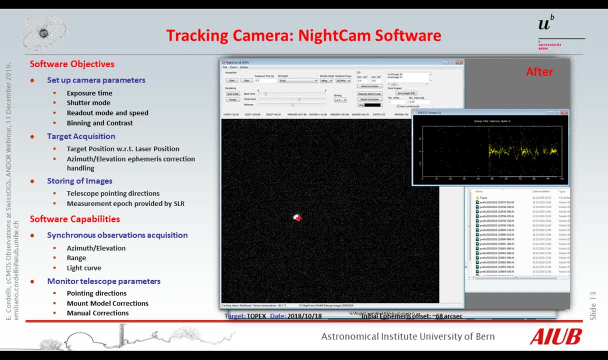 and knowing the position of the object, of the laser beam- sorry- into the camera. and seeing the position of the object, we could correct the pointing offset of our telescope, facilitating the target acquisition from the SLR system. So we needed to develop the software. 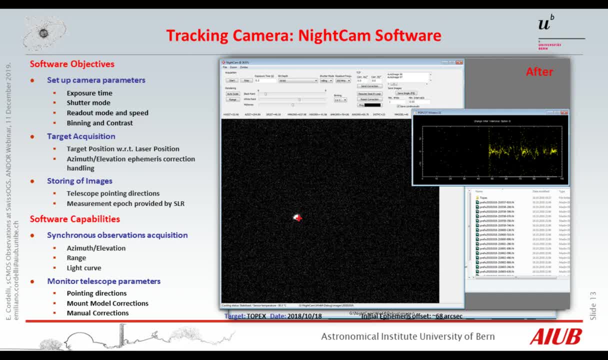 that is able to communicate with the laser software, send them correction and at the same time is able to communicate and adjust camera parameters like the exposure time, the shutter mode, the readout frequency, If you want some binning. we also implement some capability to store the images, and we will see just later why. 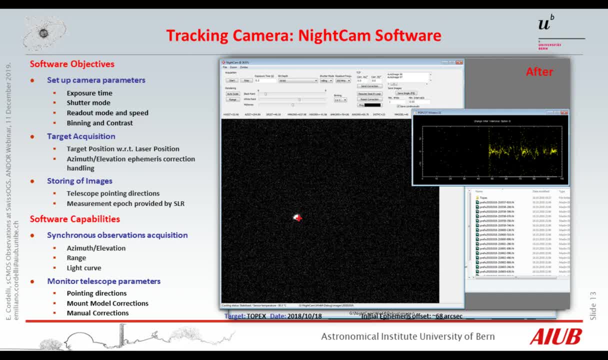 this is important. So I show you a screenshot of the software in operation. and here we have an example of the target satellite. that was TOPEX and as later I will talk quite often about space debris objects. So TOPEX, in this case and as an example of the space debris, is a defunct satellite. 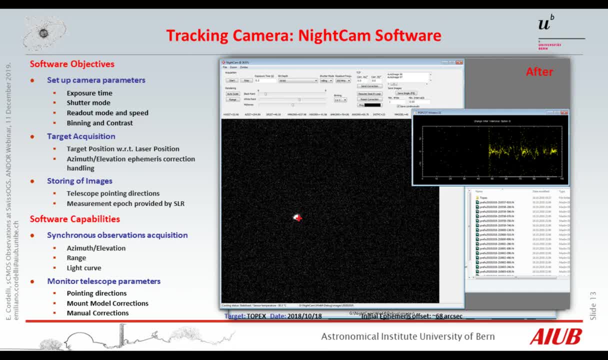 is not operational anymore and, of course, DFM rays are not accurate anymore. Actually, what we see here, we see on the red cross in the image. we see the position of the laser and we see also the position of the object as given by the ephemeris. In particular, the red cross is where the ephemeris are. 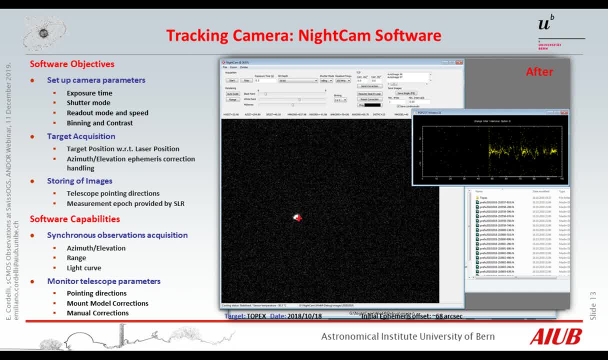 telling us to point, while the white dot is, you see, is an offset. and then we were able, by clicking on the object, to correct and align the object with the laser and, as you can see, in the small black window, we see some yellow dots. These yellow dots indicate that the laser pulse was successfully. 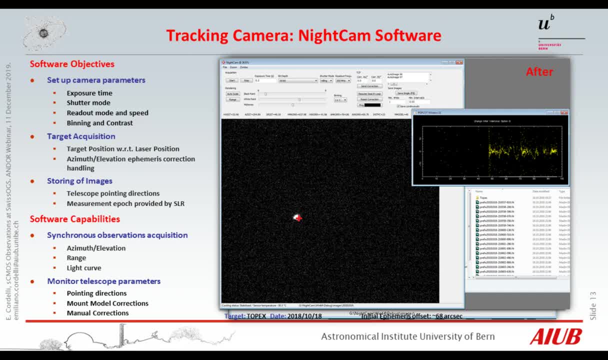 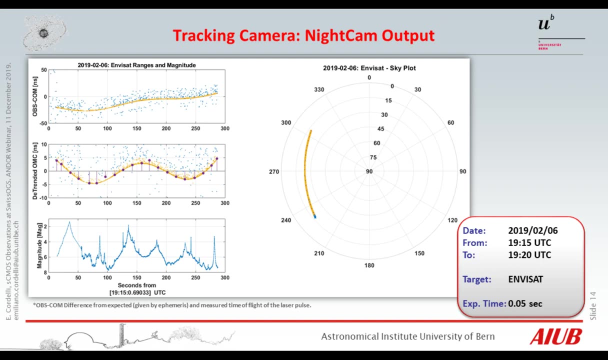 detected from the laser system, And on the background, I also show the image stored for this object. So why this is important? What is nice about this software? What we are? Okay, it's very important for us because the this software with one single 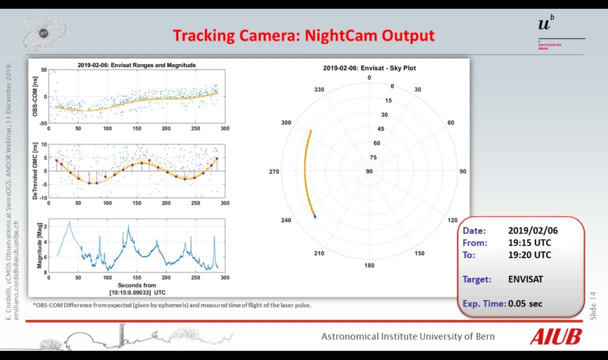 observation session allow us to get observation that can be used both for the attitude and the orbit determination of the object, And this is very important for space debris observation, Not too much for improving the laser performances, as we will see later, but for space debris observation is. 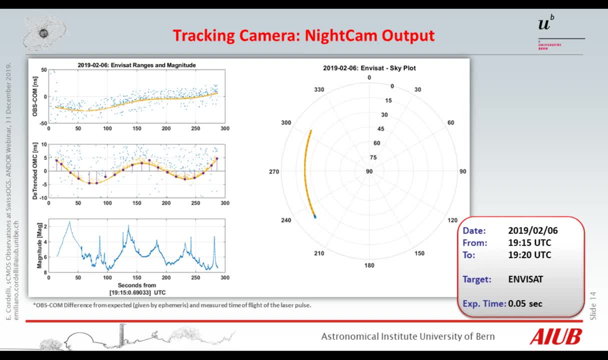 fundamental: The merging, the data fusion, especially when observing from one single station So quickly we see. these are a summary. These slides contain a summary of the observation collected by the tracking camera. We have the position of the object in the sky given by the, directly by the angular encoder of the telescope, And this: 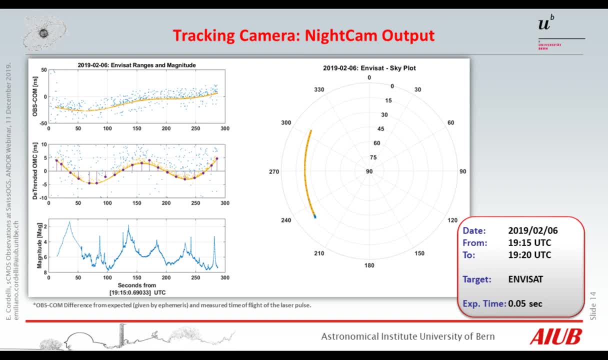 is also an advantage, Because the small field of view of the camera and the short exposure time, especially for Leo satellite, will not allow us to have enough star. They can be used for classic astrometric data reduction procedures. So we have the angular measurement and then on the top left we see the 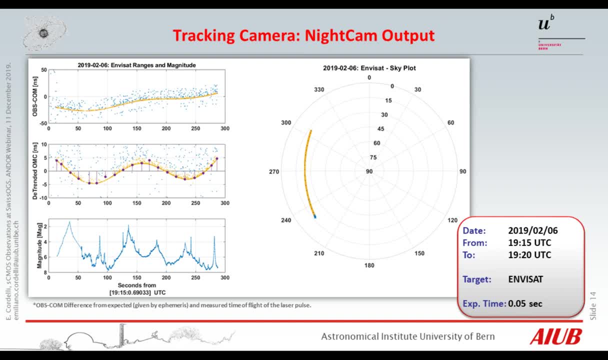 difference between the measured distance and the one measured from a distance. The difference between the measured distance and the one measured from a distance. The difference between the measured distance and the one measured from a distance, one provided by, calculated by the ephemeris. at this point, if from this distance we remove the, 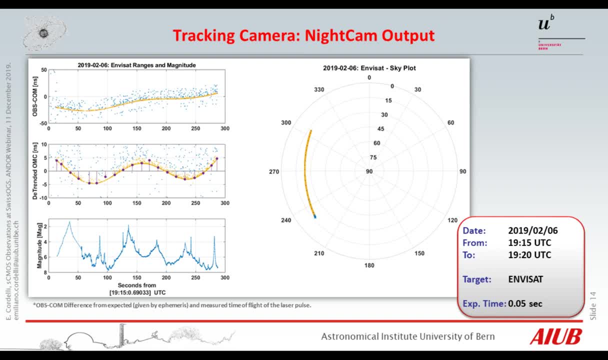 contribution of the orbital motion. we have in the middle graph, the. we are able to highlight the contribution to the measured distance given by the attitude motion, actually the, the laser measurements are very precise, let's say around the centimeter accuracy, and then we are able to range to mv, sat in this case because it can, in one of its payload is a. 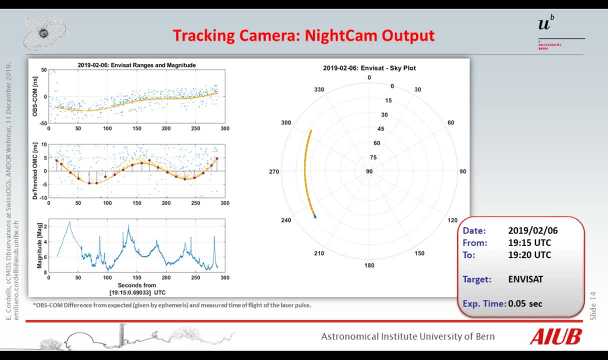 retroreflector array. this retroreflector array is not in the center of mass of the object and since the object is rotating, we see, we are able to to evaluate the rotation of the center of of the retroreflector around the center of mass. finally, in the 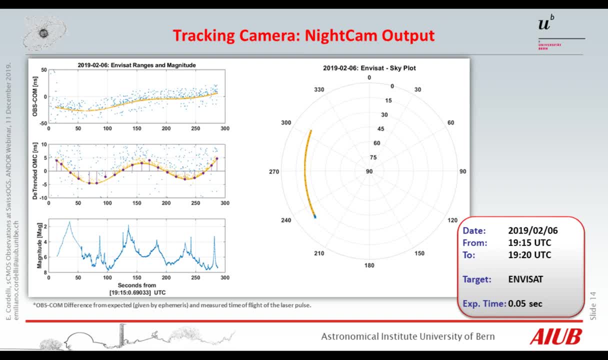 last graph, on the top one, on the bottom one, sorry- we see the results of the analysis of the images. analyzing the brightness of each frame, we are able to extract a light curve, very interesting for the space debris observation and especially for attitude debris removal operation in future. 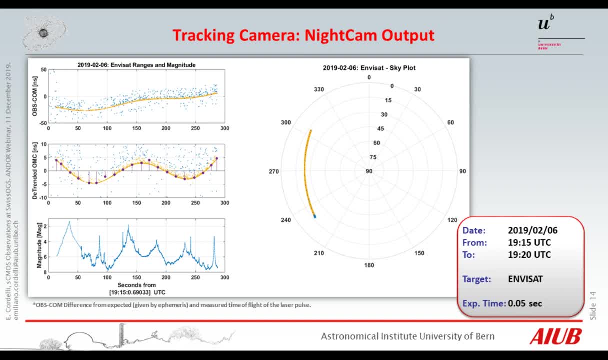 will be the attitude, the proper attitude, determination of the object. so not only the um, the rotation period, but also the direction of the rotation axis of the object, because in future, once we want to go and grab the object we know, we should know how to approach it. 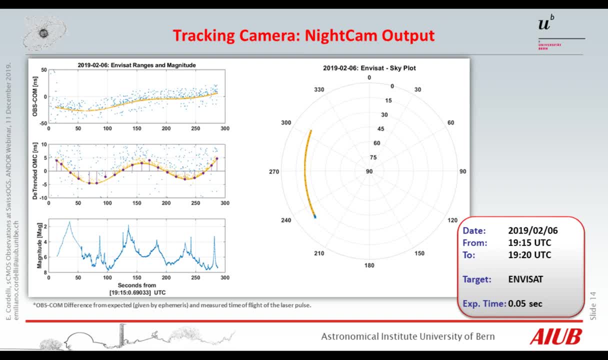 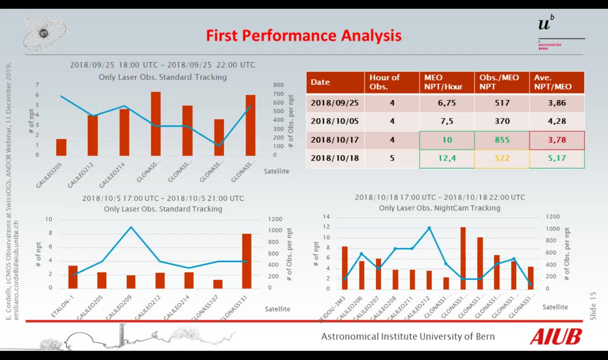 and this. both this information can be retrieved by the. there are studies to on how to retrieve this information from the data measuring, on how to retrieve this information from the data measuring ranges and light curve. then, before moving to other application, I want to show you how the performances of our laser software, of the 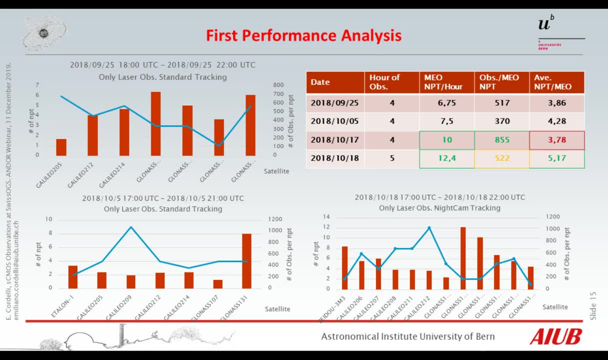 performances of the laser acquisition were improved by in the employee of the night of the tracking camera over the same amount of time. we are able to shorten the acquisition, to shorten the time needed by the system to to lock on the object. that means we are able to observe more object in in the same 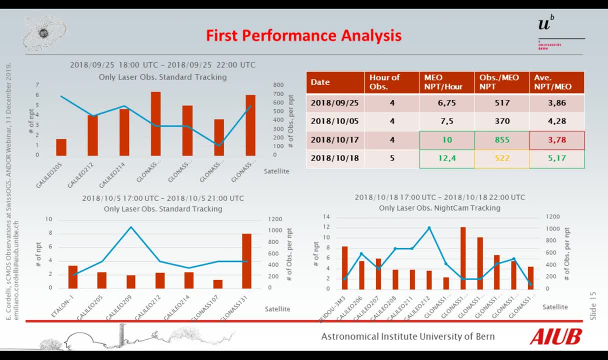 amount of time to get more observation and each observation as an higher acutely accuracy, because these we don't deliver single observation, each row observation, while we deliver what is called the normal point. the normal point is calculated by averaging the single observation, of course, the average is. 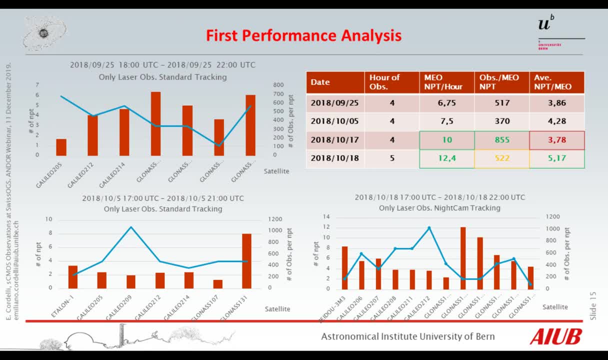 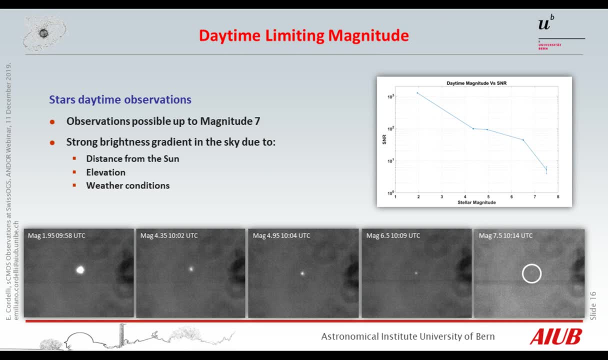 more accurate, the more the number of measurements involved. then we decided to, by accident, doing to to the direction of our step by step analysis. we did some experiments and we saw that, doing some tests, I was able to see a satellite during the day time. so I decided to do first on must and then I. 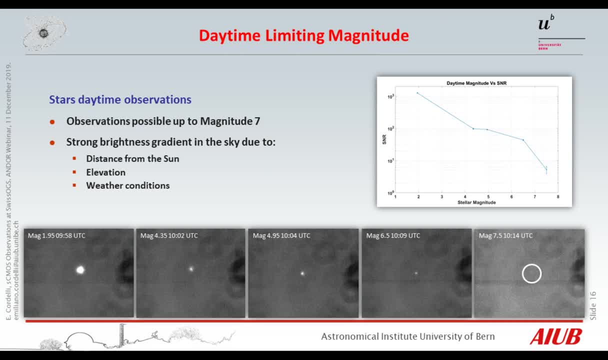 to verify that we could see Satellites during daytime. and then I did. we did to the faintest on the right and that confirmed the math that I did and we are able to see up to magnitude 7 during full daytime. Actually, these pictures were acquired at noon. 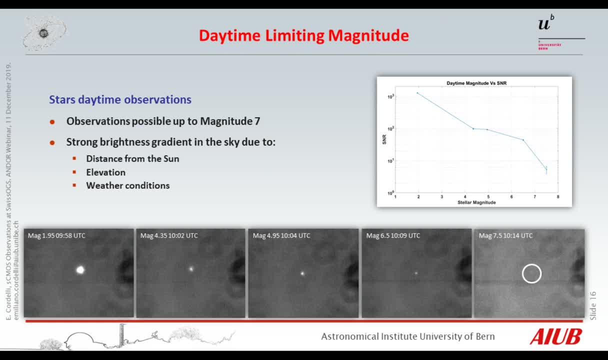 Something that makes the daytime observation a bit more difficult are the strong brightness gradients in the sky. Toward the horizon, the sky is brighter than at the zenith, and of course the brightness of the sky depends a lot also by the distance from the sun. 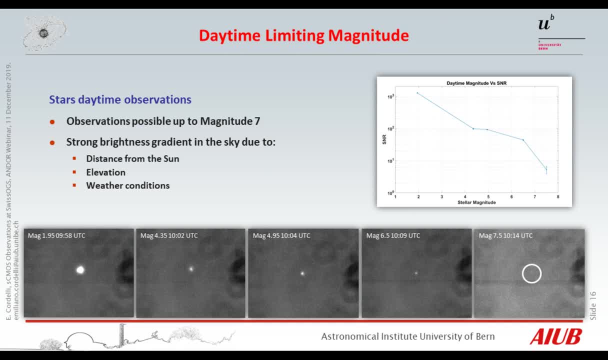 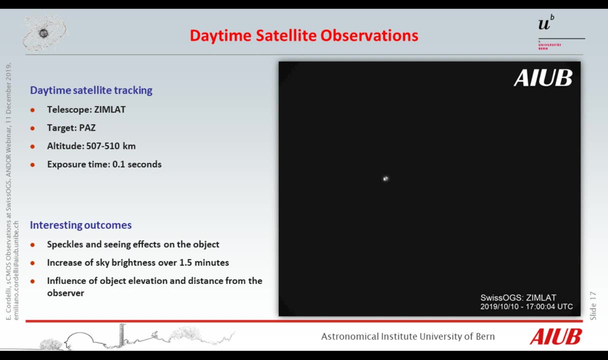 and from the weather condition, A dry day is better than a humid day. Then, okay, we verified that we are able to do something during daytime, so I decided to do some tests over satellite. Here we have just a GIF that I created using 20-25 images acquired for this satellite. 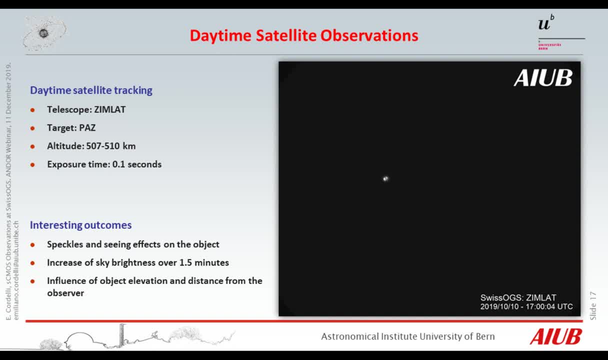 This is a standard satellite laser-ranging target and this was observed with 0.1 seconds of exposure. This is the image of the satellite around the sunset. What is interesting from this image is that if we look at the object, we see that the object is not always point-like, but is changing. 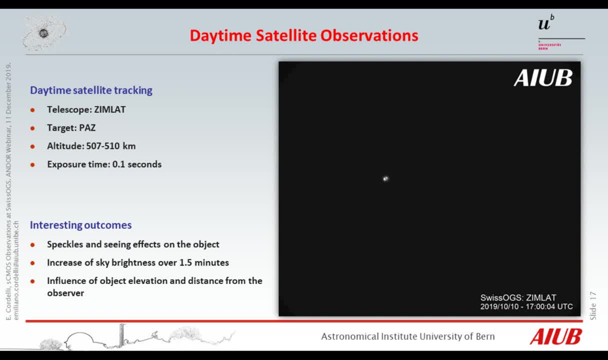 These are the effects of the seeing, atmospheric seeing, and in principle one could do also some research about the speckles that we see. Then what is interesting is the how the sky break ground is the brightness is increasing very fast. 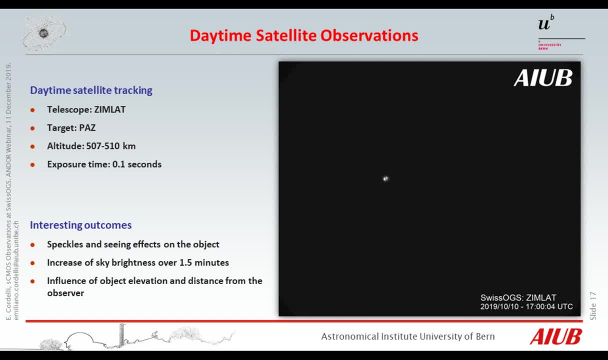 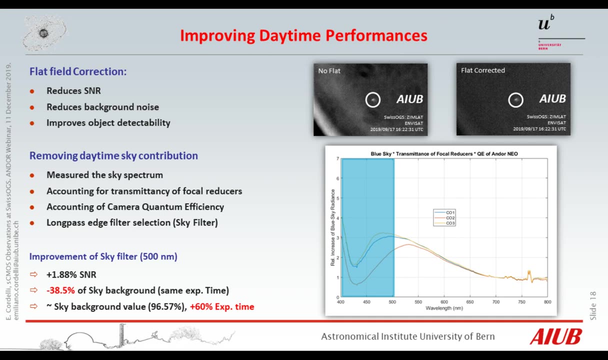 over one and a half minutes of time interval between the first and the last image. The- the sky background. the sky during daytime act as an homogeneous source of light and this homogeneous source of light at the end was showing. and this homogeneous source of light at the end was showing. 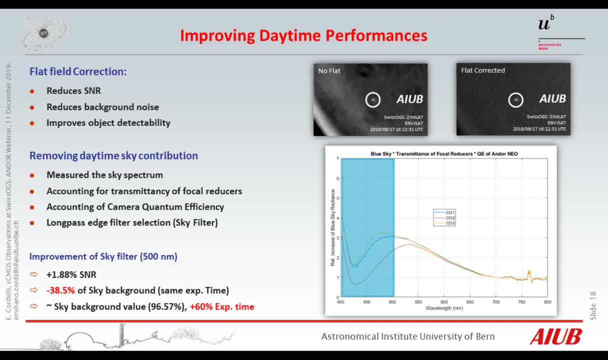 and this homogeneous source of light at the end was showing some, some dark spots on the camera. This is not on the camera, it's not due to the camera at all, but this is simply dust on the focal reducer. 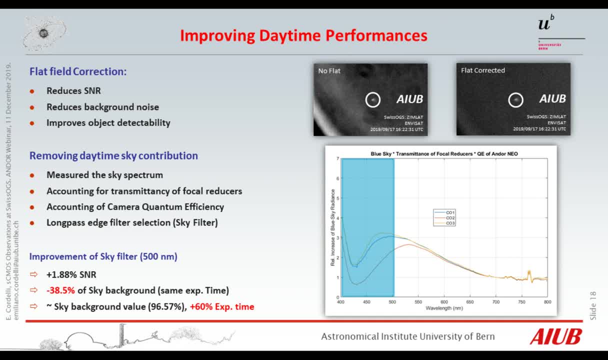 So to improve the quality of the image, especially the one acquired during daytime, what we can do is flat-fielding of the image. This allows us to remove some vignetting and also the effect of the vignetting and also the effect of the vignetting. 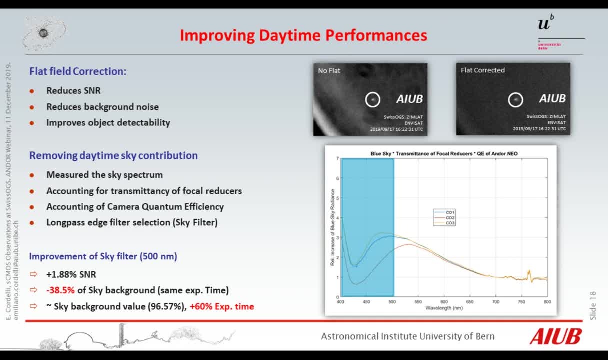 of the vignetting and also the effect of the vignetting of the dust, and this improves the detectability of the object at the same time. also to improve the performances during daytime, we decided to analyze the sky spectrum, take into account the transmittance of the focal reducer and the camera quantum efficiency. so we have everything is. 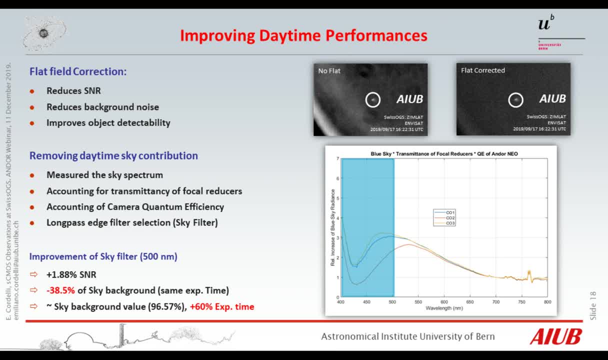 summarized in the plot over here, and this is uh, the, the radiance of the sky all over the the visual spectrum. so in order to improve the the performance during daytime, we decided to insert the long passage filters with the cutting edge at 500 nanometers to cut out. 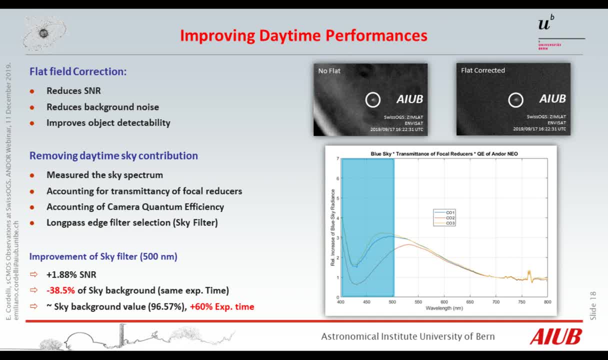 some of the blue light of the sky, and this allowed us to increase the signal to noise ratio on the same source, reduce the sky background flux by something about 40 percent, and these translate directly into an increase of the exposure time that can be used to detect smaller objects in the sky. so now let me talk about some. 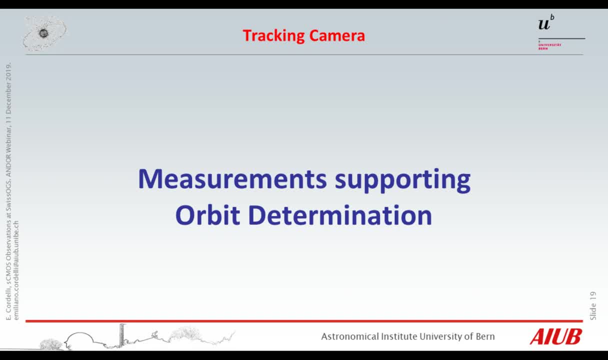 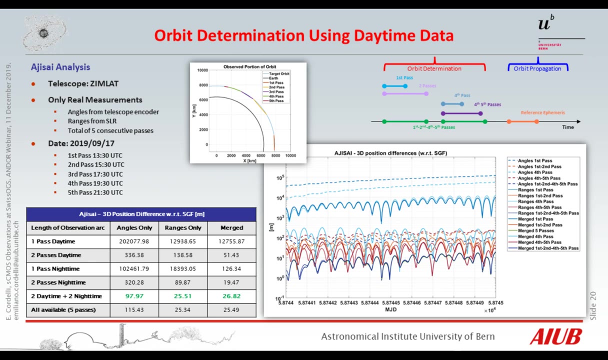 one daytime observation. why the use of the of the tracking camera and the use of different kind of observables is important for the orbit determination, especially if we talk about space debris. so what we? i? we performed some tests. we um acquired the observation during one and two passes. 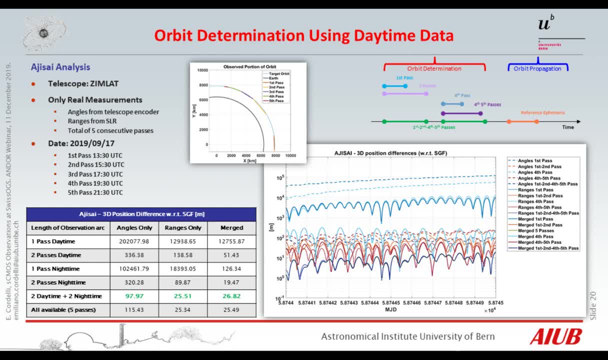 during daytime and one and two passes during nighttime. and then we compared what we can get in terms of accuracy um processing separately one, two passages processing separated, the daytime observation with respect to the nighttime observation, then putting them together and then we played also on the kind of observables that we are um that we are collecting um using the 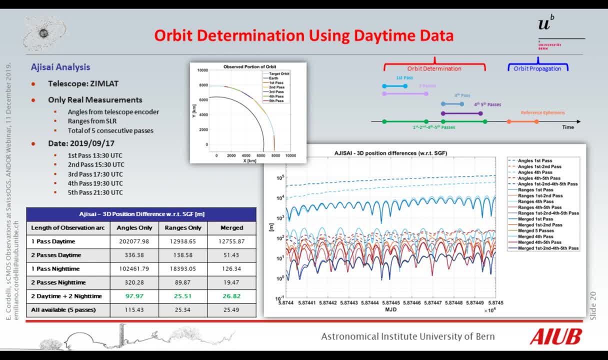 tracking camera, uh. the first analysis was done on a gsi, i decide, the standard target for the laser community, and this allowed us also to have some reference orbit against which i could compare my orbit determination result and essentially what we can see is that the effect of the merge, merging of the data fusion, can be seen, especially for 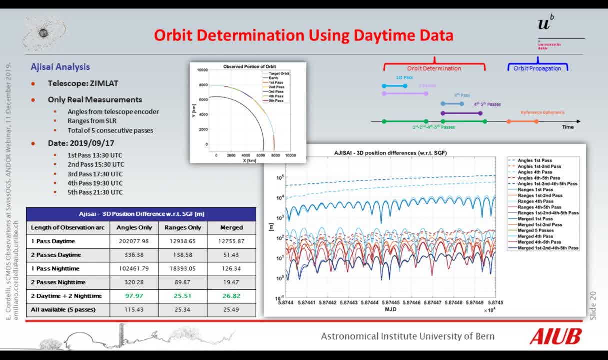 the one pass case for the nighttime. one pass case. if we use only angular observation, we will have an error over four days, an average error of 100 kilometers, while if we use merged data the error reduces to 130 meters. then if we now, instead of using only nighttime observation, 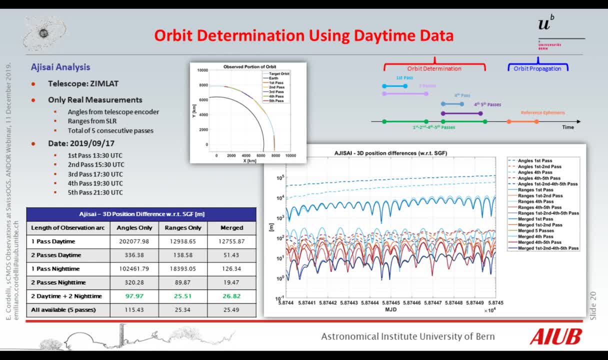 during classical space debris observation, you can rely only on night time observation, since the southern light has to be illuminated, the object has to be dominated, but the observer has to be into the shadow because the actually this is the limit of the technology, this is a limit of the ccd cameras: that they cannot. 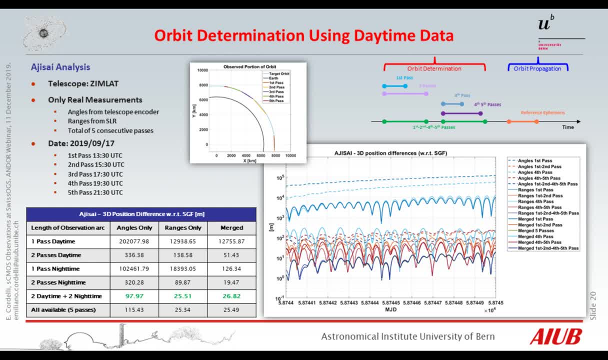 go for very, very short exposure time due to- for us, as an example, is a problem. the problem is caused by the external mechanical shutter. it is solved by the CMOS that use an electronical shutter. then one last comparison that I want to show you is the improvement given by the merging daytime and nighttime. 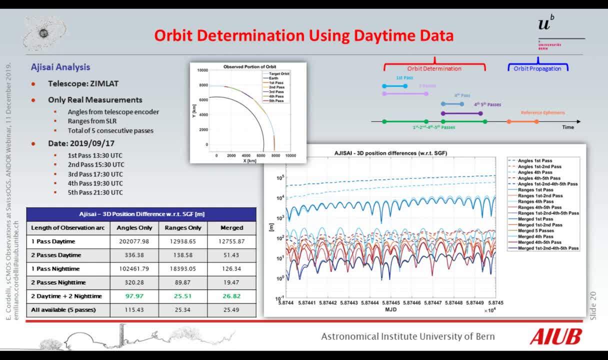 observation, and this is visible from the small plot on the top where we can see that the green and red segment are the is the portion of arc that usually we can observe. if we rely only on night time observation, standing the observation to the daytime, we are able to observe almost a quarter of an. 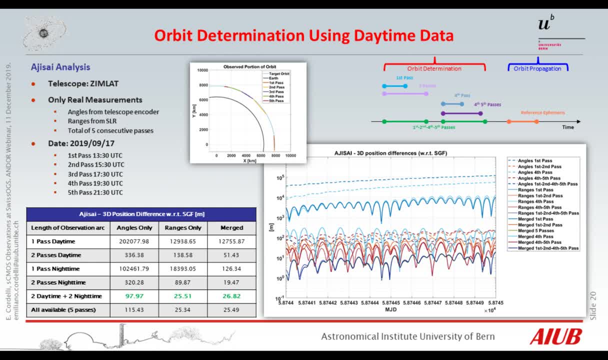 orbit and this is translated directly into night time observation, the orbit determination accuracy. if comparing one passage during nighttime we have an accuracy again 100 kilometer that reduce to 100 meter even processing only angular observation. if we put together daytime and nighttime passes, the best solution that we got was 27 meters over of average error over four. 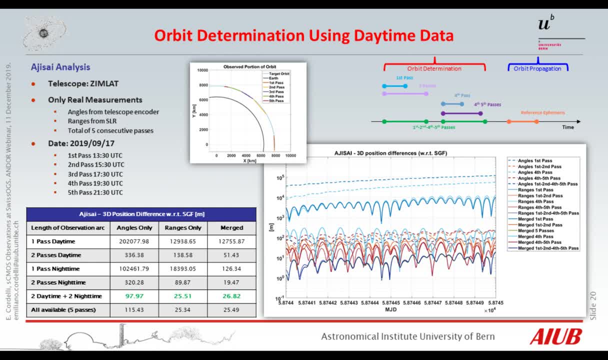 days of provocation, and this is quite important for space debris activity, since before this kind of observation we didn't have any a priori information about the orbit, so we could really perform in what is called an initial orbit determination and then a successive orbit improvement. that allowed us to reduce the 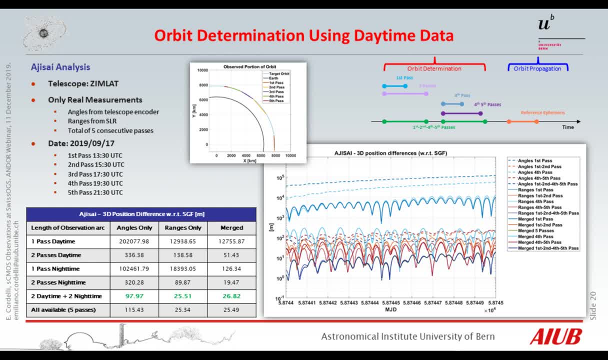 covariance and the uncertainty region of the object position to a radius of, let's say, 20, 30 meters. this is important for collision avoidance maneuver the. the space is crowded of space junk that are very dangerous for the satellite, since each and every particle contains a very high energy that could potentially destroy our mission. 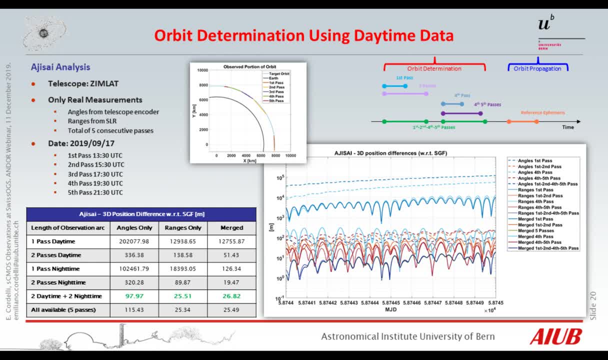 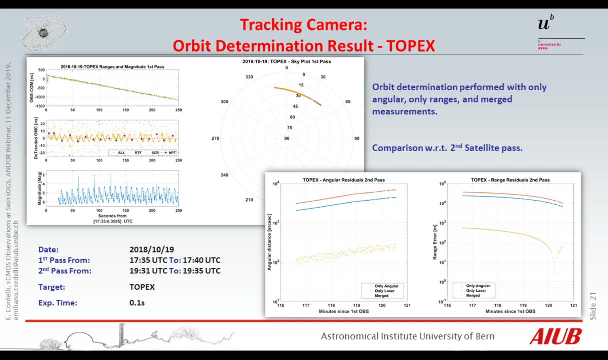 knowing precisely where these objects are reduce the non necessary maneuvers and enlarges the lifetime of the satellite. okay, but is you're telling me- yes, you use the satellite- that we know already which orbit which is his orbit? so we decided to perform some tests also to understand the space debris. Yes, so the space debris. it's typically a bunch of liquid objects that I've been able to get up into. space debris is a bit. Since it didn't have any any reference orbit for this object, I needed to observe it in two consecutive passes. I used the measurement collected during the one past to determine an or bit that was propagated and compared with the observation collected during the second pass of the satellite. Always use our tracking, niemandly but to determine in orbit that was propagated and compared with the observation collected during the second pass of the satellite. Always use our tracking. humanitarian information is still gonna be used, so 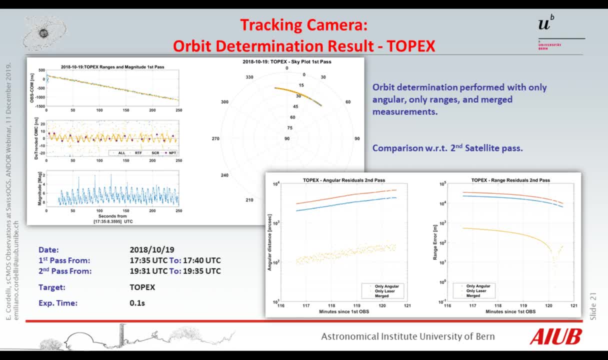 camera. so here, what we is interesting to see is the on the left plot. we see the rapidity of the attitude motion and, as we will see later, this object will rotate with this, with the rotation period of 10 second, and is still spinning up and this 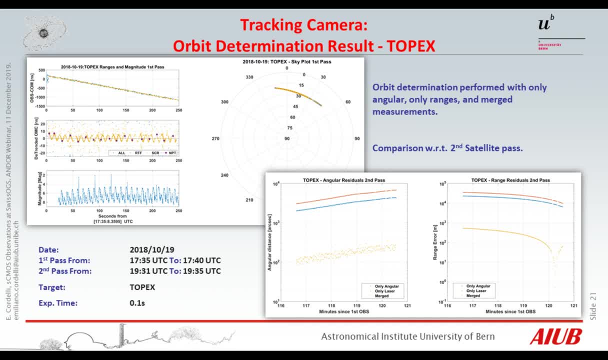 speed is also increasing. and then what is interesting to see is that, using merge measurement, we can improve our orbit determination accuracy in, by word, one order of magnitude if we look only at the angular position. by two order of magnitude if we look at the estimation of the distance between between the 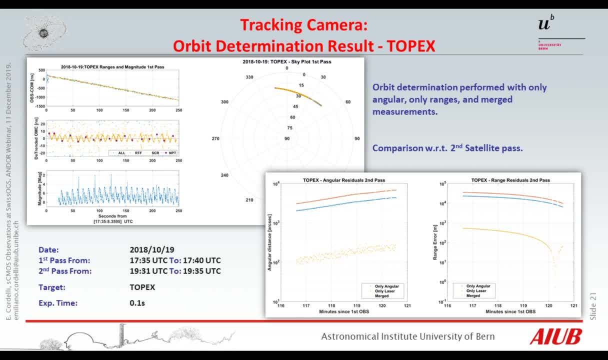 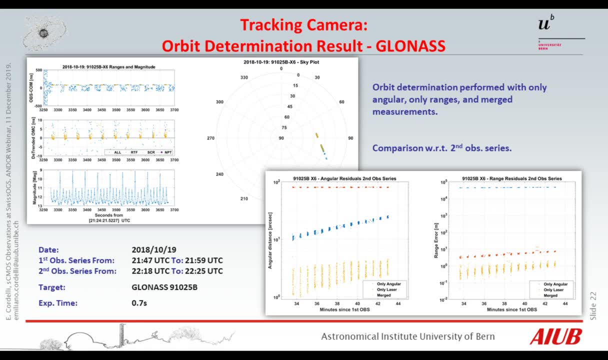 observer and the object, but is again, these are low earth satellite. we could also prove that we were able to range also to I altitude satellite. this is the results. are these observations were collected to a debris that was former a glonass satellite. this satellite is orbiting at around 20,000. 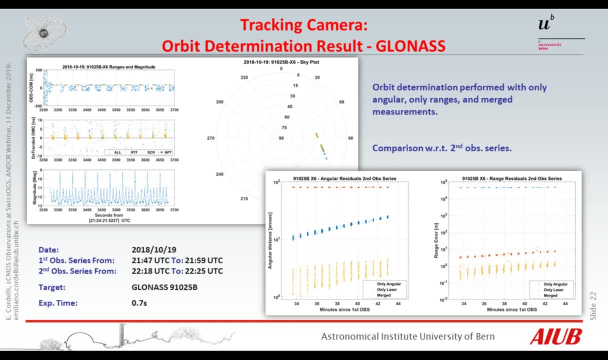 kilometers and, okay, the improvement using merged with respect to homogeneous measurement is less evident, but because we in the distance between the two series of observation is smaller in time and these two series of observation belongs to the same path of the satellite. what is interesting from the left plot is the position of the good equals, the. 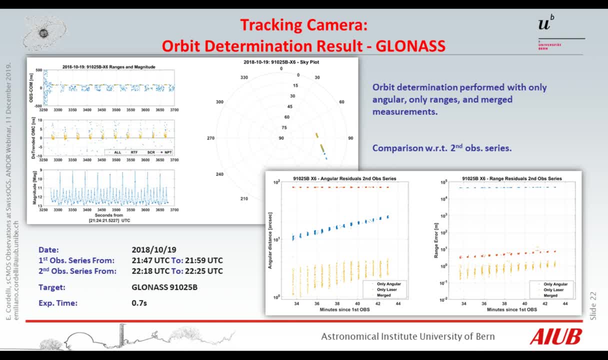 yellow point of the laser with respect to the light curve that we are observing. actually the light curve shows some pattern, but from the battery itself we are not able to determine which part of the satellite we are currently observing, and this information is provided by the lasers. we know that the reflector 40 said the light is in the body phase of 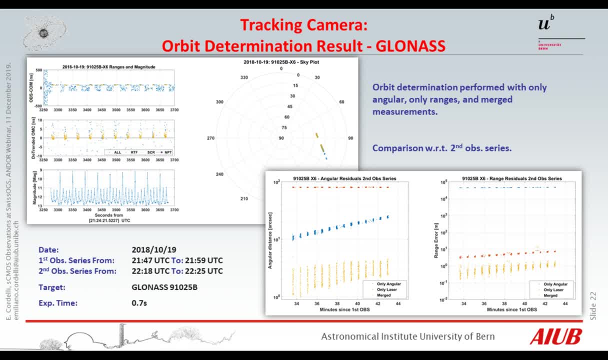 the satellite means that they yellow is a�� region. I mean the portion of the light curve that correspond to the yellow region of good egos. this is exactly the nadir phase of the satellite. Why it is digression? because this led me the connection to the measurement that can. 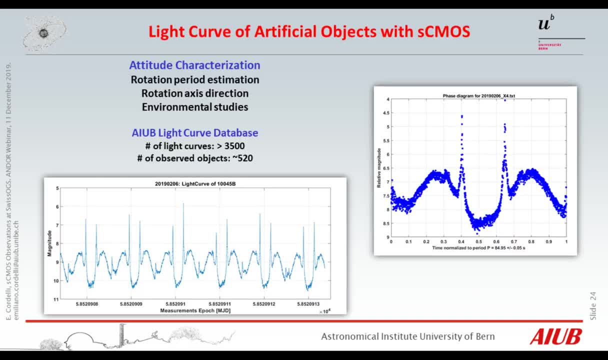 support the attitude determination. actually knowing which is the nadir phase of the satellite, we are able to to to perform what is called a three-axis orbit determination. Why the orbit determination is sorry, three-axis attitude determination. why the attitude determination is important again, for is important for mainly for active debris removal mission, where we have to know. 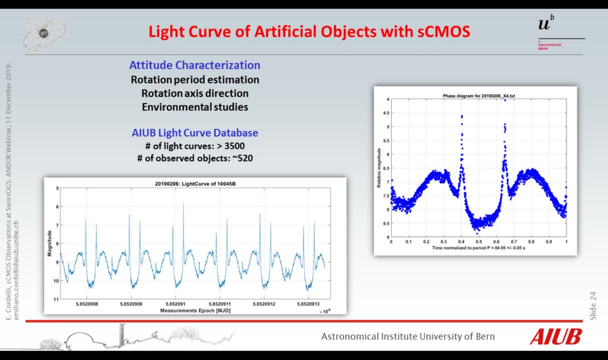 from which direction is better to approach the satellite: to grab it to the space debris, to grab it and pull it down, or if we can do also some environmental studies here. in this slide I showed you the light curve acquired, the high-resolution light curve acquired with CMOS camera using half of a 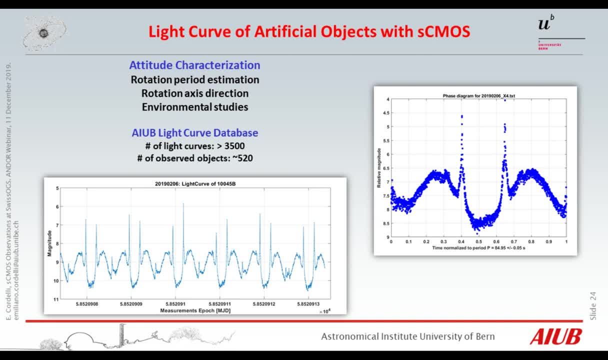 second of exposure we were able to discriminate some specular reflection given by the peaks that we see in the light curve of this rocket body is a rocket body can be assumed as a cylindrical shaped object. so if we analyze the assuming that this object is in a flat spin condition, the rotation 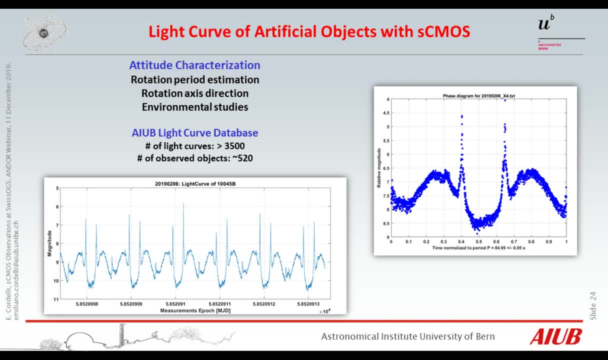 should produce a brightness variation that looks like a sinusoid, and this is exactly what we see here. if we exclude the maximum of the peaks given by the specular reflection and these relative minima, that probably is caused by one of the sides of the rocket body is difficult. 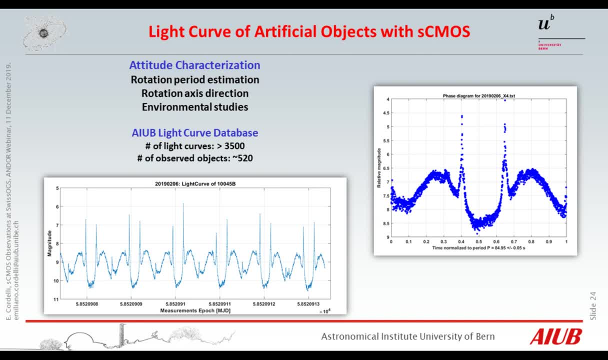 from the light curve itself to discriminate which is the nozzle and which is the adapter side of the payload. but what is important is that from this measurement we can extract the rotation period as for the asteroid, and in principle, knowing also the shape of the object, one can infer also the direction of the rotation axis. these two data 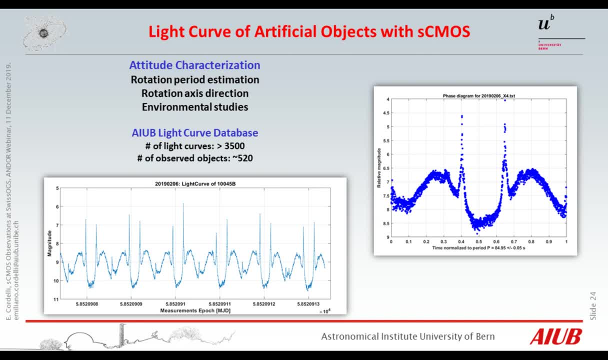 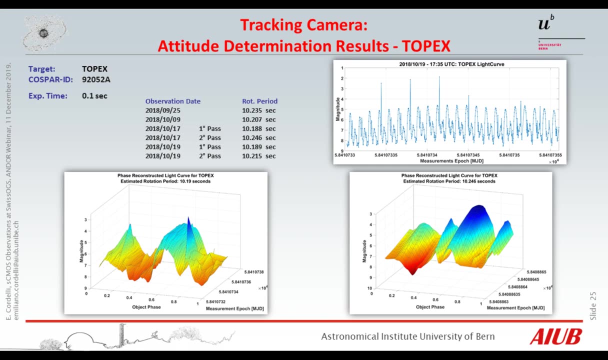 could be used to do also some environmental studies of, to evaluate what are the torques that are acting on a space, on a spacecraft, and the current relationship between the end frame and the subsystem. so the raise of solar energy will have moregew functionEL well. So 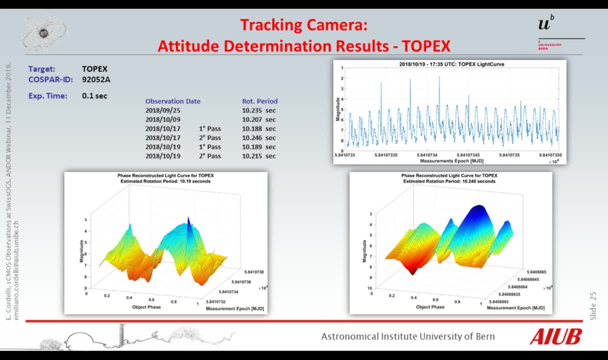 if it's, it's everybody is getting its lên. well, let me SUS: position of the object with respect to the Sun and the observer is important because, in relation with the altitude motion, the light reflected toward the observer is different. This is exactly what we see here on the bottom plot This: 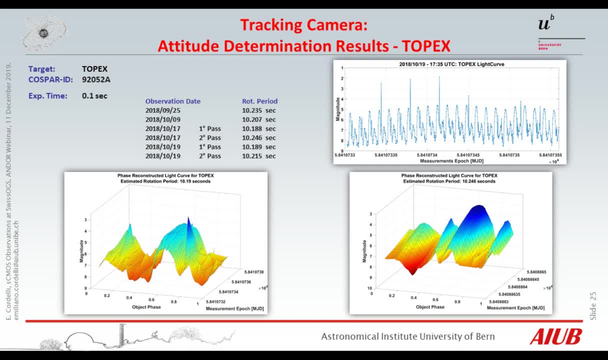 is the same satellite, acquired in a time distance of two days. The rotation period is pretty similar, but in the first case we see relatively flat behavior over the path. We have only in a portion of the path some specular reflection, while on the second path we have an increase of the brightness due 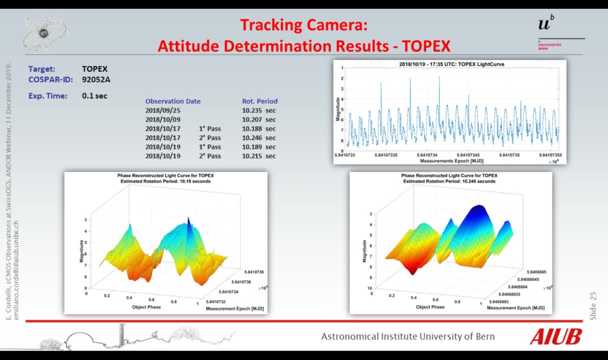 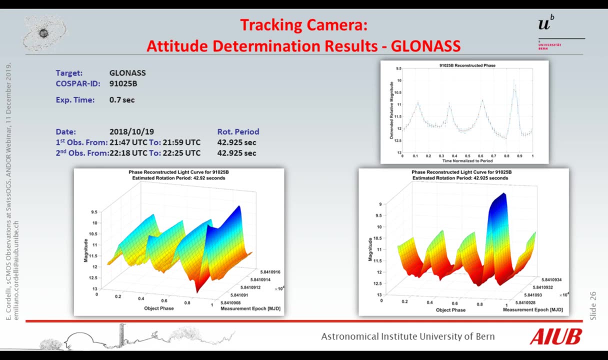 to the reduction of the phase angle, and even if the target satellite is the same, the features shown in the two plots are quite different. The same is valid for the higher altitude satellite. We used the exposure time at 0.7 seconds. this time and again, this is. 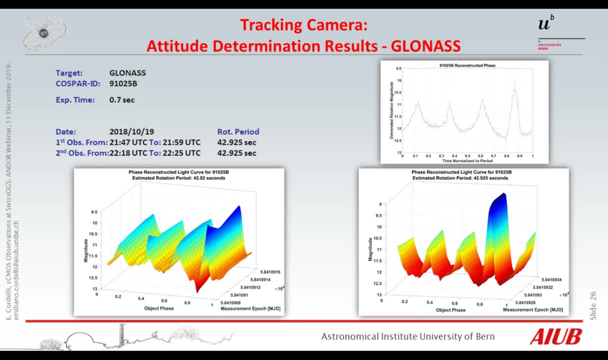 the same GLONASS as before. so the two series of observation were acquired with the distance in time of 20 minutes roughly and we can see that the effect of the change in the observation geometry On the second part, on the right plot, we see a higher. 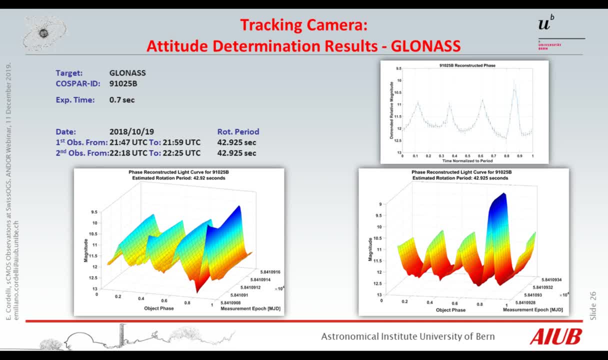 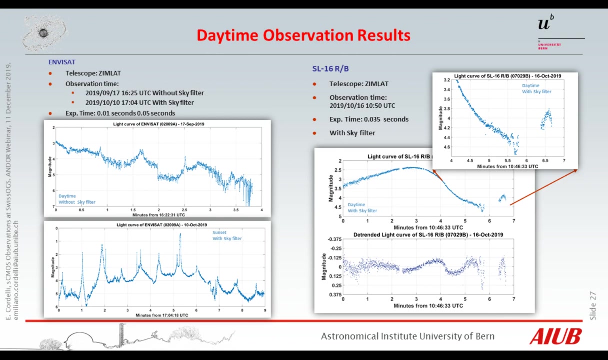 difference, a bigger difference between the absolute maximum and the relative maxima of the light curve. But what is interesting now, what we can do during daytime. the observation geometry and illumination condition change pretty fast During daytime, And then here I will report some results acquired really. 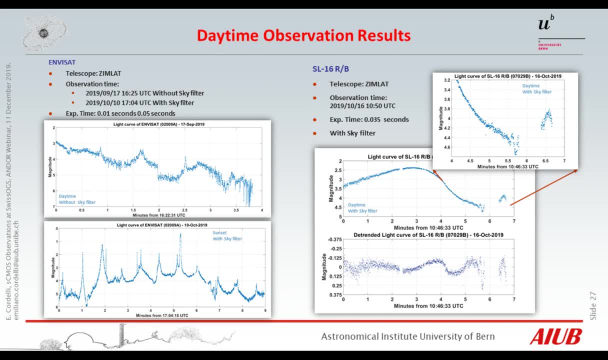 during daytime. On the left side of the slide we see the results obtained for for MVSAT during daytime and during the sunset. During daytime we didn't yet use the sky filter, so the light curve is pretty noisier. Nevertheless, we have some features. 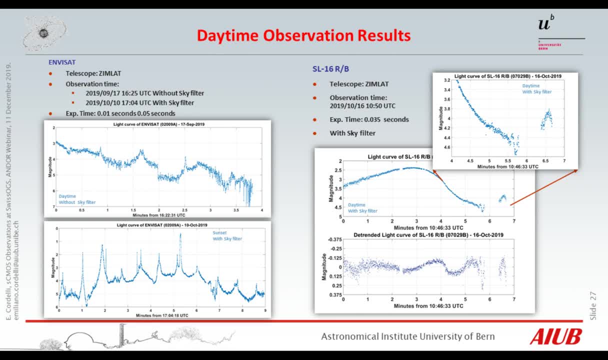 that can be identified also into the second plot. A second example on the right side is obtained for a rocket stage. Again, this is a cylindrical object that should be- should- rotate around its maximum axis of inertia. This is an assumption that we can do, since in the past we used the maximum axis of inertia and not the maximum axis of inertia. 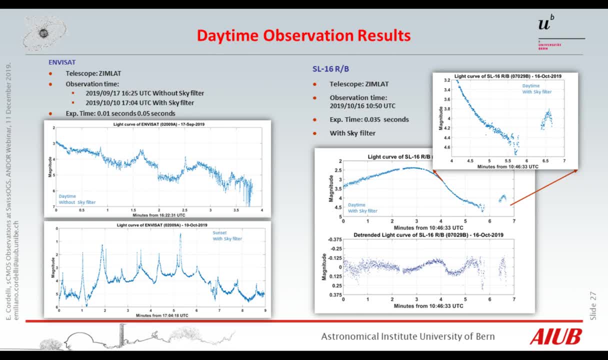 the space. there are some dissipative torques that let the object migrate from the spin around the minimum axis of inertia toward the maximum axis of inertia. what is interesting here is the change of the observation condition in relation to the attitude motion we see at the beginning, the 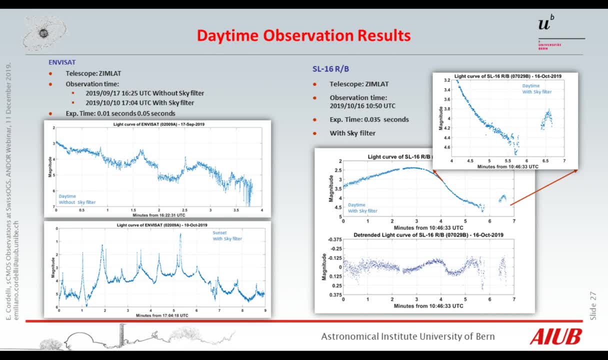 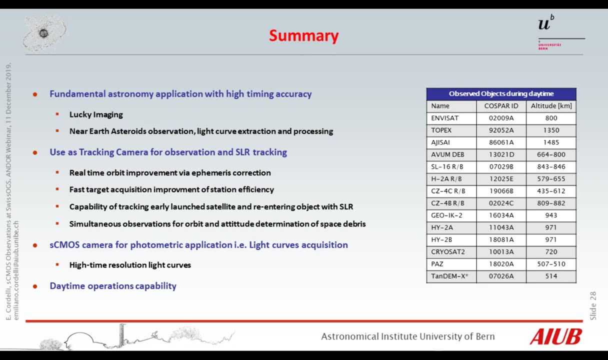 light curve is pretty flat, but then toward the end some features start to appear and start to be amplified, and this is exactly the contribution in the reflection given by the attitude. so that brings me to the summary. so the CMOS camera were used for a huge variety of applications. 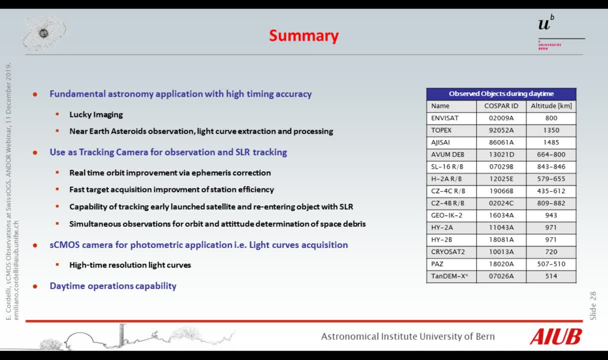 from the liking images to the observation of asteroids. we used the tracking camera for support in support of the. we used the CMOS camera as tracking camera in support of SLR observation. this allowed us to get observation for the simultaneously for the orbit and the attitude determination. 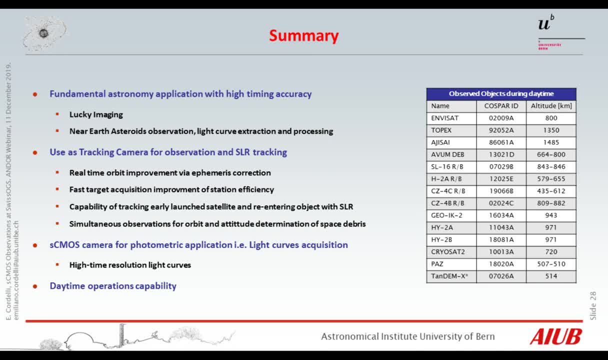 this is important because this kind of camera could allow us to track objects that are either yearly launched or which are re-entering in the atmosphere, where the ephemeris are of poor accuracy we were able to track. the camera allowed us to um to observe a light. 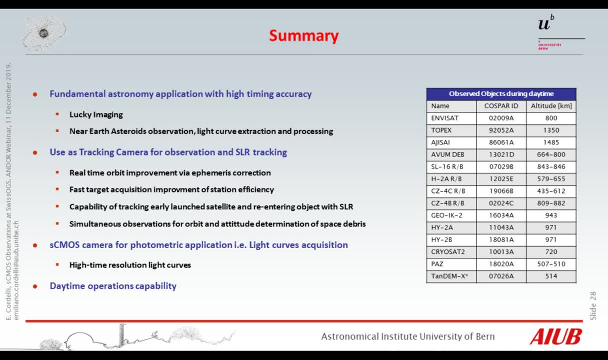 curve with an extremely high resolution. that is usually it's not possible with ccd camera. and finally, we were able to extend our observation time also during daytime, and this is in the table. i just put a summary of all the objects. that varies from satellite to rock. 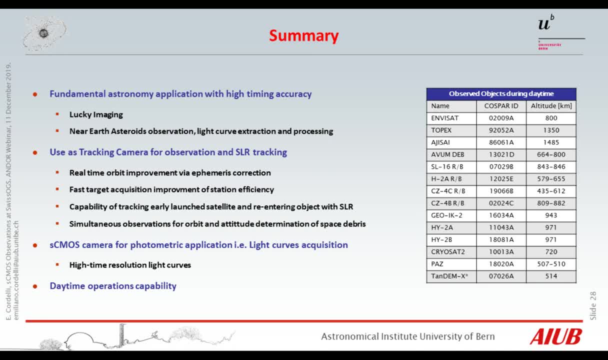 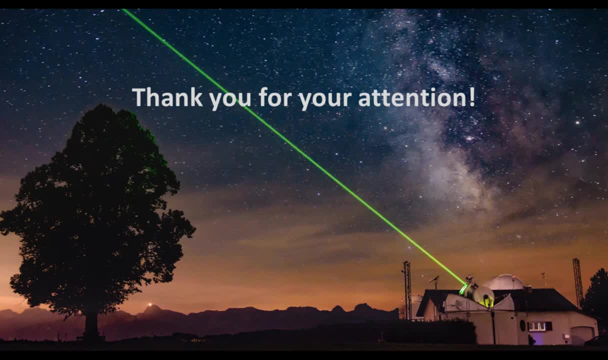 and this is in the table. i just put a summary of all the objects- that varies from satellite to rock, at different altitude that we are able to observe only during daytime. so that brings to that's everything from my side and thank you for your attention and thank you. 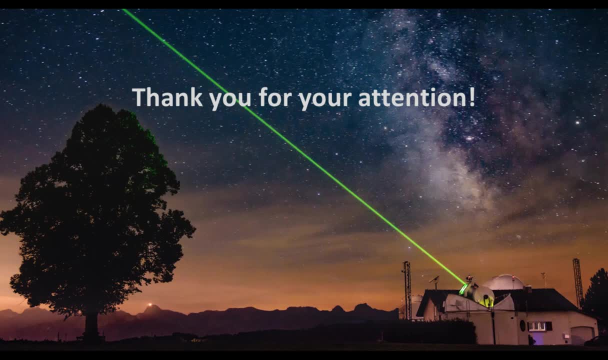 Kristy for the opportunity. thank you, Emiliano, for that informative presentation. now kicking off the second part of our webinar today is Dr Inez Yuvan-Bollier. Dr Yuvan-Bollier is an astronomy specialist at Andor. 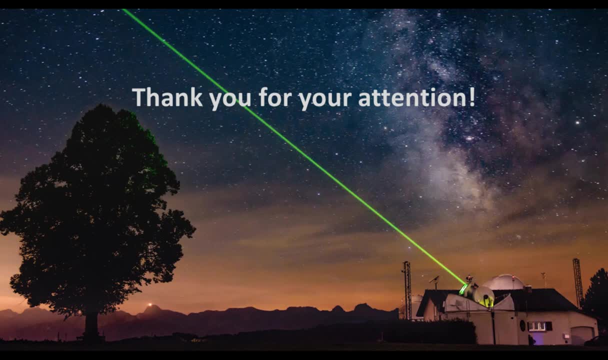 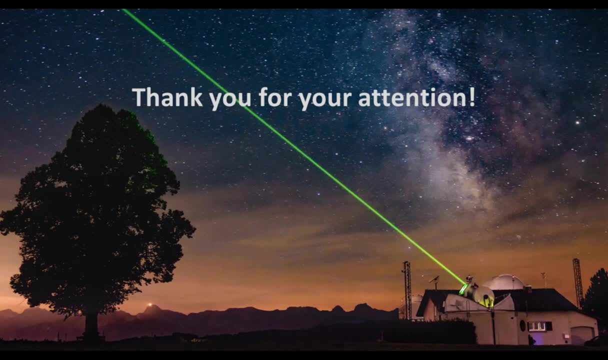 she studied physics, with a primary focus on astrophysics, at the university of graz in austria. in april 2018, she completed her phd thesis in multi-color photometry of transiting extrasolar planets. in addition, she has held a research position at the space research institute in graz. 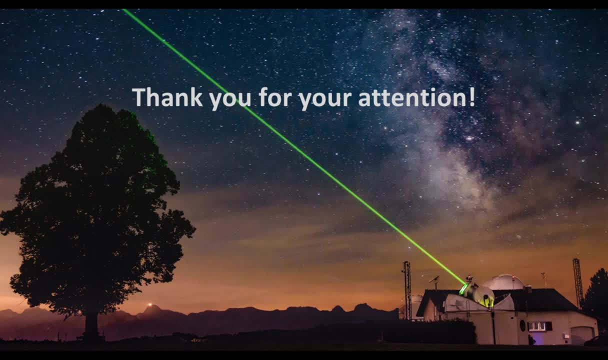 and spent some time lecturing at the university of indsburg. for a complete biography on dr yuvan-bollier, please visit the biography tab at the top of your screen. thank you, christy, for the introduction and thank you, emiliana, for talking about the observations. 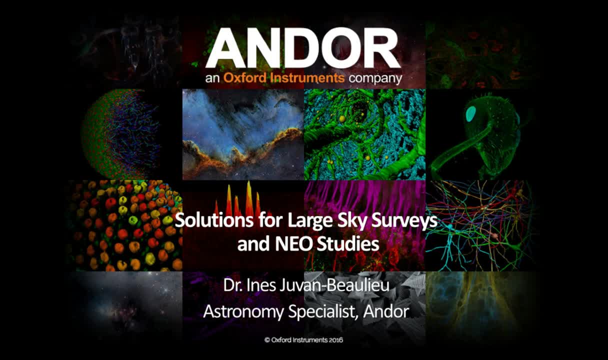 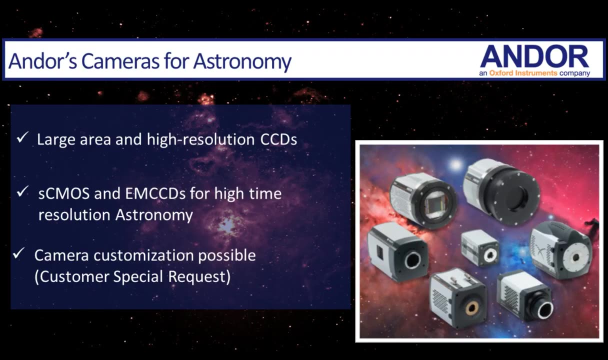 ines. you may now begin your presentation. so thank you, christy, for the introduction, and thank you, emiliano, for talking about the observations that you perform at the timar vault observatory. so my part is now to talk about under joins camera solutions for large sky surveys and near of object studies. so at 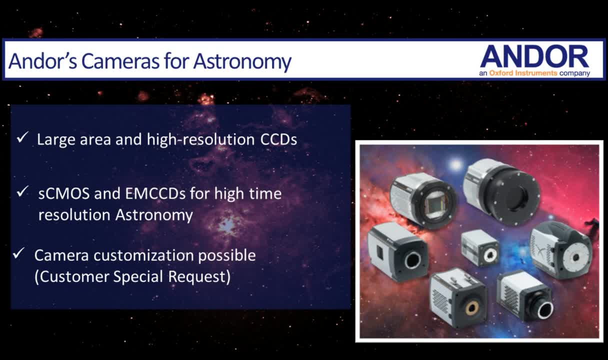 first i would like to talk about under camera solutions for astronomy in general. so we have variety. healing depends a variety of options. we would Anders Cammerz solutions for many people around us, but you become aβ studyinguminator in throughмы, so that is newcom. 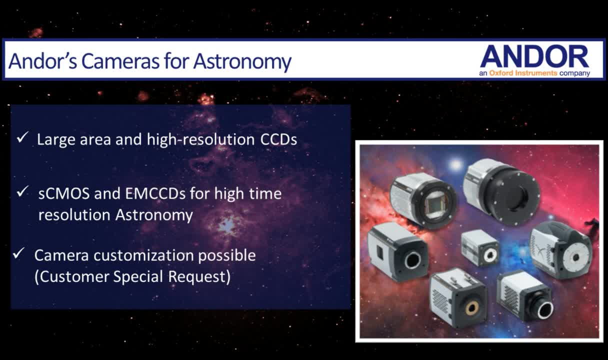 we offer large area and high resolution CCDs. Then we also have SEMOS and EMCCD camera solutions, especially for high time resolution astronomy or if you have to deal with low light conditions. So in that case EMCCD cameras would be the perfect solution for you. 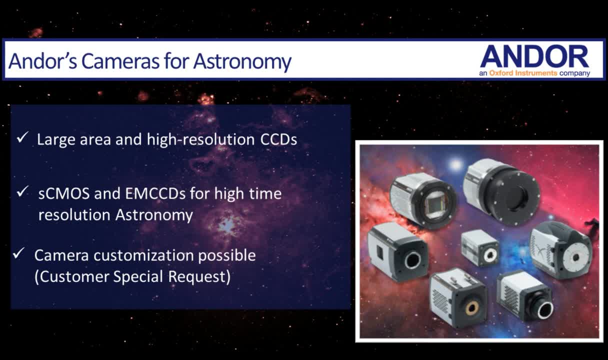 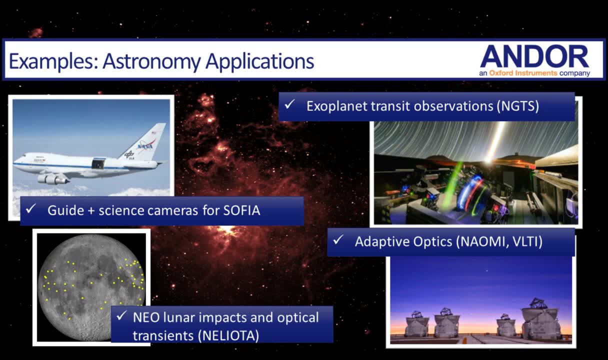 And also I would like to highlight that we do offer camera customization. And just so you have an overview of which projects UNDOR is involved in, so which projects use UNDOR cameras? We have, for example, our EMCCD cameras. 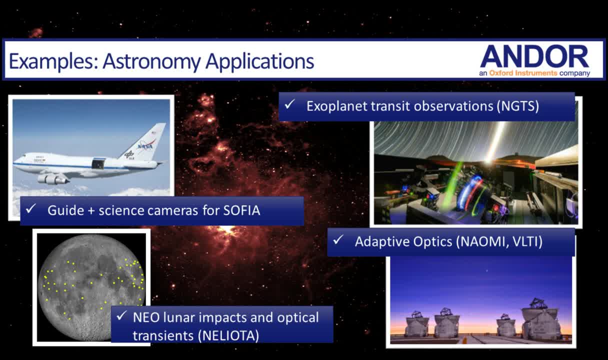 called the Ixons used at the SOFIA telescope. So there they're used as guidance and science cameras. Then also UNDOR cameras are used for exoplanet transit observations, like, for example, the NGPS survey. There they use several ICON-Ls. 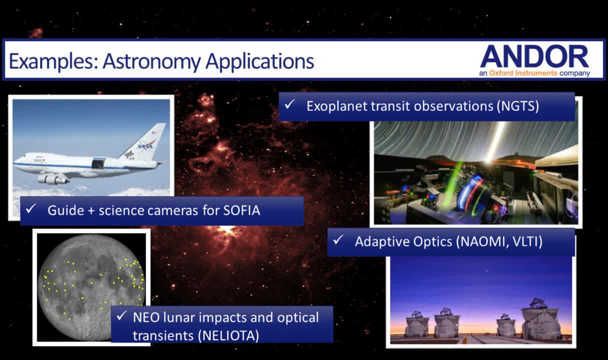 which are also customized. so those are 2K by 2K CCD cameras. Then we have two Xyla cameras. Those are SEMOS front illuminator cameras used for the NEBIOTA survey. So that means near-Earth object, lunar impact. 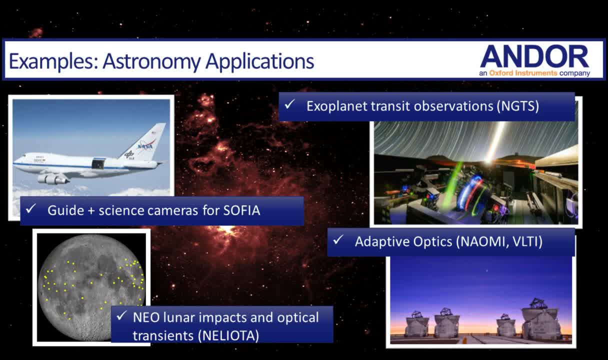 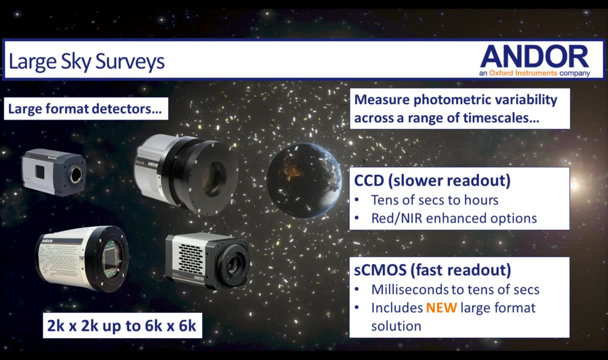 and optical transient studies. And then we also have several Ixon EMCCDs used for adaptive optics projects like the NAOMI project at the BLTI. But now I'd like to come back to large-sky surveys. So if you perform such surveys, 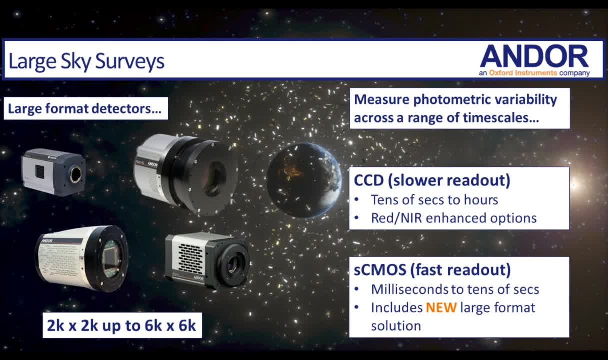 I would recommend to use large-format detectors. That is because you can make use of the wide field of view that you can achieve. So for that, we offer 2K by 2K detectors. up to 6K by 6K detectors. 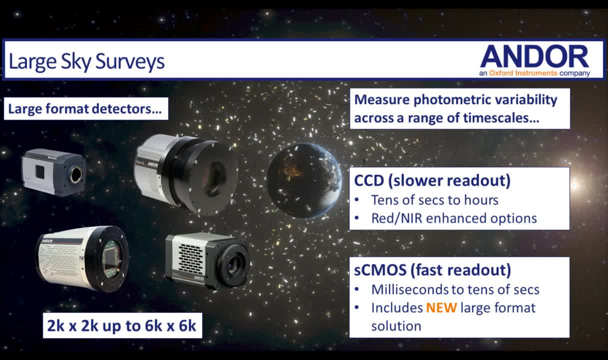 and that really offers you the possibility to measure, and that really offers you the possibility to measure and that really offers you the possibility to measure photometric variability across a wide range of timescales. So, for example, if you work with CCDs. 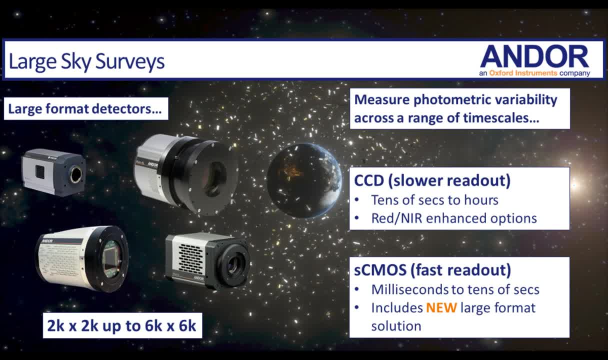 that operate with a slower readout to maintain a lower noise floor. that is really great if your exposure time is in the range of tens of seconds to hours, And also our CCD options offer sensors with enhanced options. So that is really of advantage when you want to observe. 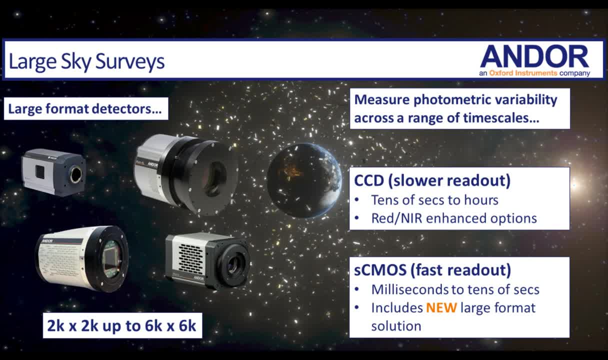 So that is really of advantage when you want to observe. So that is really of advantage when you want to observe cool objects. And then if you require high-speed observations so you observe astronomical phenomena that change quickly or that change quite fast, then your exposure time is in the range. 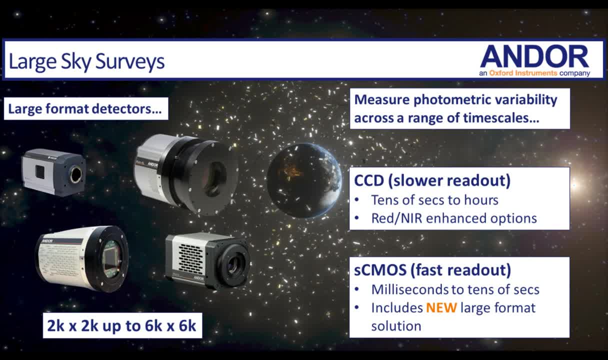 of milliseconds to tens of seconds. Then we at CMOS is the technology that I would recommend and that you also see. on the bottom of the image, on the left, you have a 4K by 4K sensor called the BALOR, And then on the right, next to it, is our back illuminated. 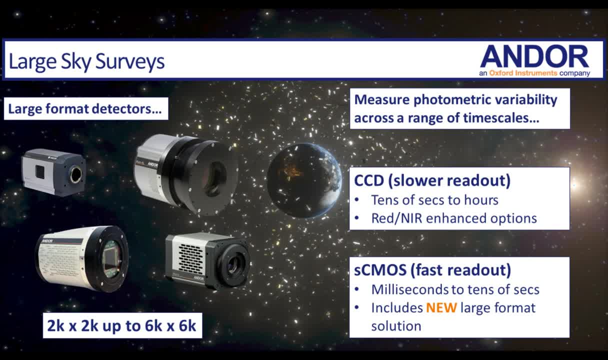 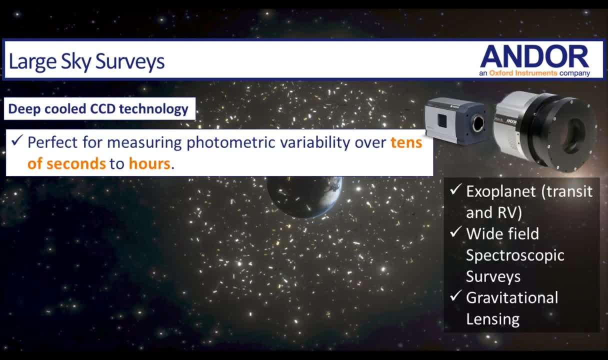 2K by 2K at CMOS camera called the MAZANA, And I will also talk about our new large format camera solution called the BALOR, which you see there on the left and on the next slide. But I would also like to highlight again. 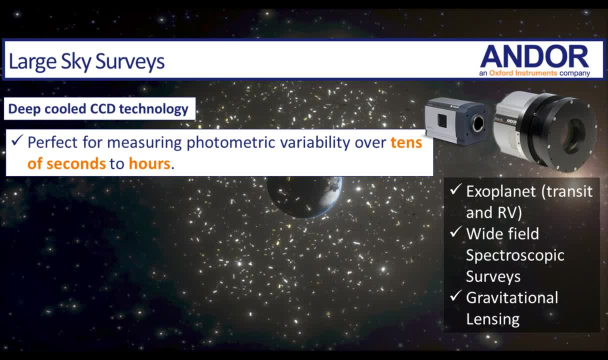 our deep-cooled CCD technology. So, like I said, this is great if you're exposed in the range of tens of seconds to hours. those cameras are mostly used for, you know, exoplanet observations, for example, if you use transit or RV method. 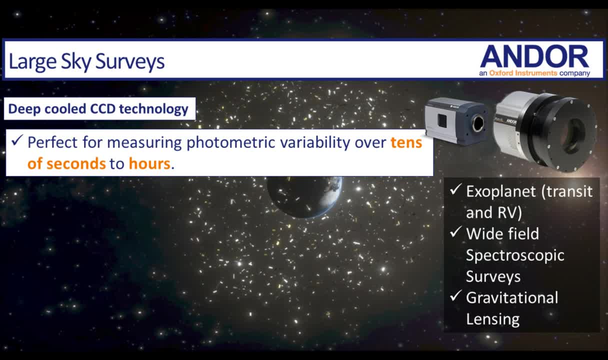 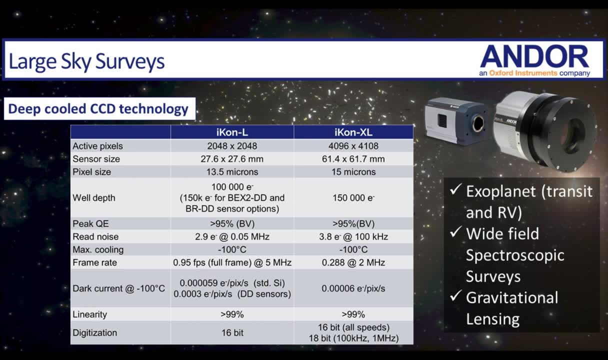 then also in wide-field spectroscopic surveys and for gravitational lensing. Now I would like to present to you some specifications of two of our CCD cameras that we offer. We have here the Icon-L and the Icon-XL. The Icon-L is a 2K by 2K device. 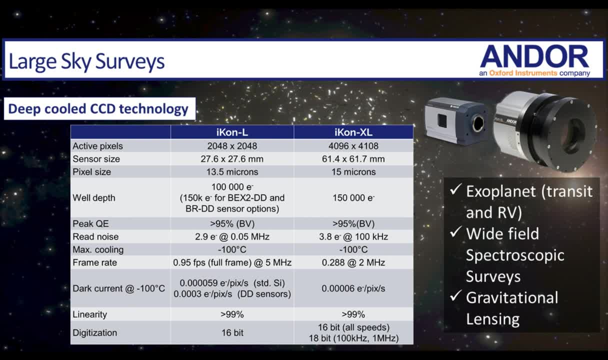 whereas the Icon-XL is a 4K by 4K device. They slightly differ And they offer a very low read noise. So if you go to the Icon-XL site, what you see here that through our deep cooling down to minus 100 degrees Celsius. 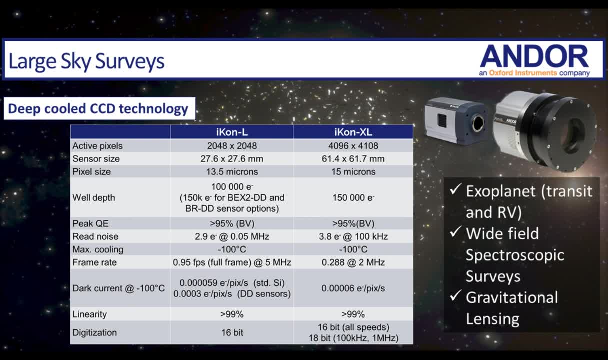 we do offer a very, very low, dark current value. You see it here: for the Icon-XL, for example, a value of 0.0006 electrons per pixel per second. And also we really offer a low read noise of about 2.9 electrons or 3.8 electrons at 100 kilohertz. 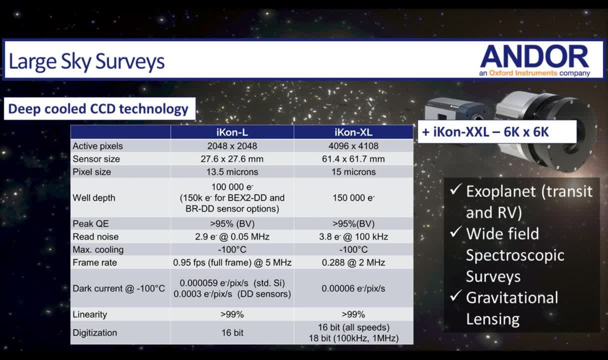 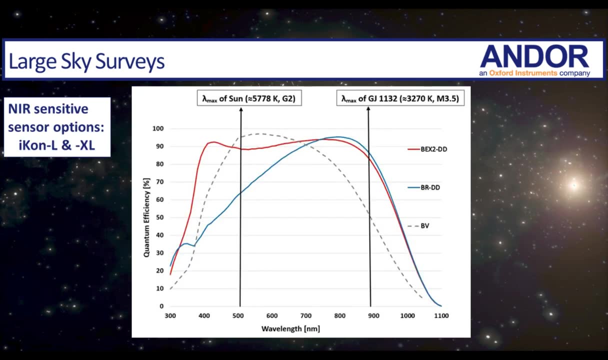 And also what I would like to highlight is that we do offer an Icon-XXL as well. This is a 6K by 6K device, so that's even bigger than Icon-L and Icon-XL. All right, so here on the slide. 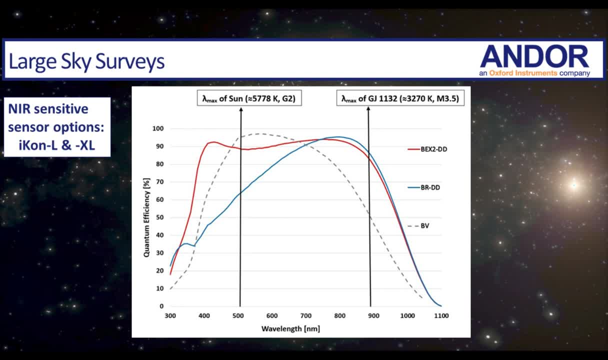 I would like to mention the different sensor options that we have for the Icon-L and Icon-XL. I mentioned earlier that we do offer near infrared sensitive sensors. So you see this here in the plots. You see the quantum efficiency plotted with the wavelength. 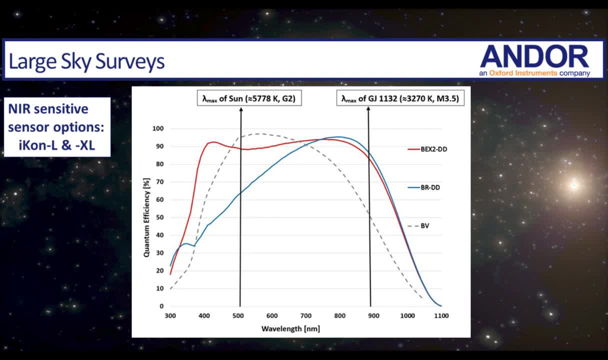 And there we have a comparison of three different sensors. One of the sensors is the BV, That's a standard visible sensor implemented in those cameras. And then we also have deep-degraded sensor options which really offer this extended near infrared sensitivity. So it's called the BRDD and the VX2DD sensor. 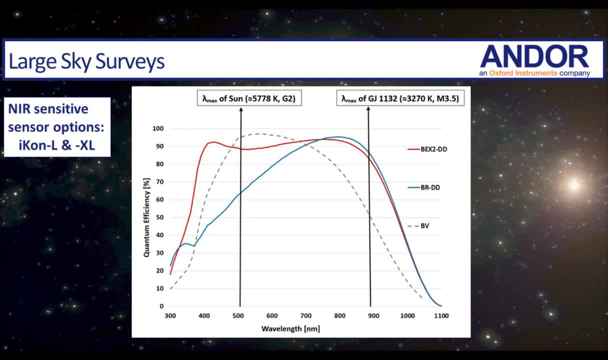 And also the VX2DD sensor has another coating on it, and that means that we also have an extended sensitivity in ultraviolet. And on top of this plot you also see the peak emission of the sun compared to the peak emission of an M-type star called TGA1132.. 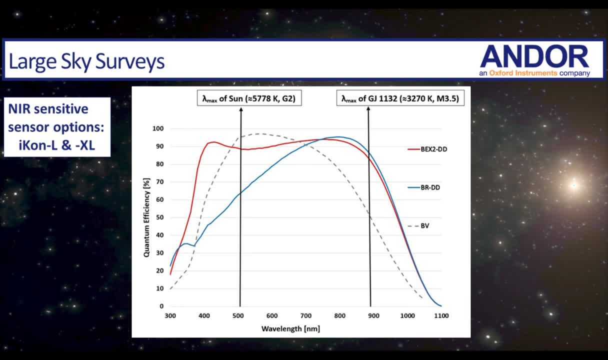 So this is the coolest star. So the peak emission, peak wavelength of this star would be just below 900 nanometers. If you want to observe cooler objects, you would really go better with a sensor option, But you also have the ability to see a lot more. 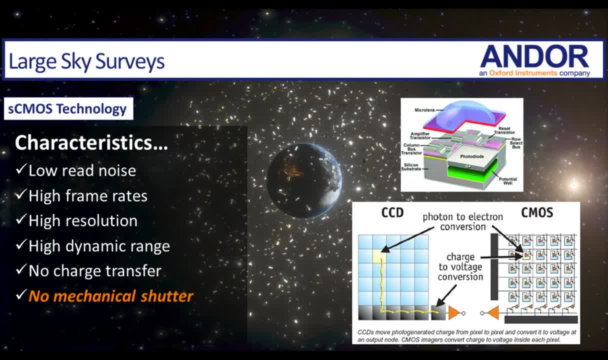 of the amount of energy that is near infrared sensitive. Before talking about our S-SIMOS solutions for large sky surveys, I would like to highlight the benefits of S-SIMOS detectors and the technology. So what are the characteristics? These types of detectors offer a low read noise. 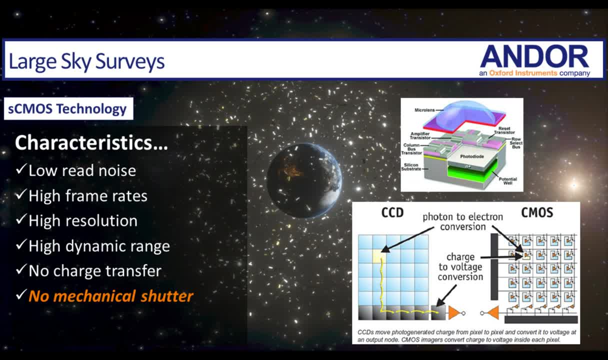 while simultaneously allowing to image. with high frame rates, You can achieve a high resolution. They allow for high resolution dynamic range. there's no charge transfer and, on top of that, they're not using a mechanical shutter. so this is a great advantage if, for example, you're observing from remote locations, where 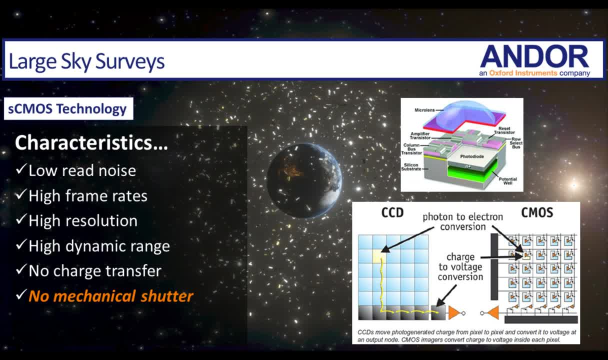 it's not easy to exchange a broken mechanical shutter, so as seamless detectors work with electronic shutters like, for example, rolling and true global shutter. and all of these characteristics and benefits of a cmos detectors come basically from the sensor architecture. so you see, on the right hand side in the image, a comparison of the sensor architecture between ccd and cmos cameras. 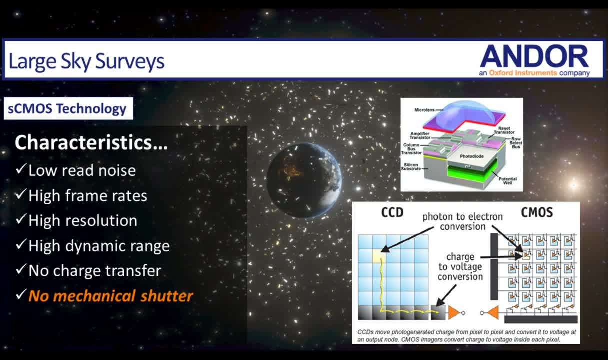 you have here marked that the charge to voltage conversion on a cmos sensor takes place at each pixel, whereas in ccd the charge is shifted from pixel to pixel and then converted to a voltage. so because of that, because of these differences, cmos detectors can offer these specific characteristics. 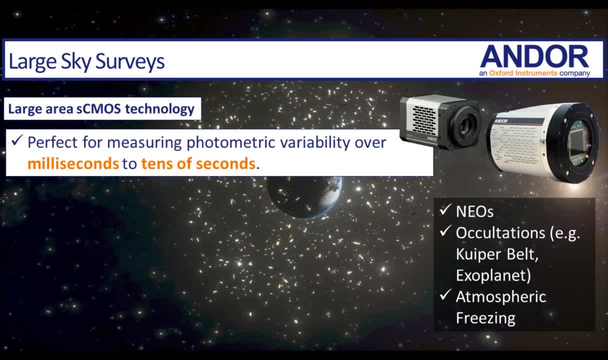 and then i would like to highlight our sdmos camera. so again, this is great if you want to observe, uh, with an exposure time of milliseconds to tenth of seconds. so this is usually applicable if you do near, all near of object observations or occultations, for example, corporate belt objects or even exoplanets. and it's also great if you want to. 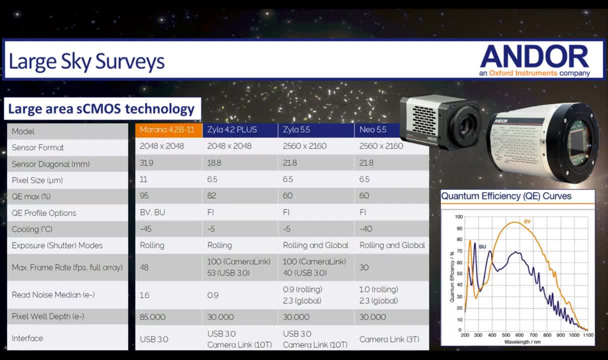 do lucky imaging or specular imaging, so here's an overview of some of our cameras that we offer. you see in orange, this is the marana. it's a 2k by 2k back illuminated s cmos device, you really reach a peak quantum efficiency of about 95 percent. i have to pause, given here on the right hand side. 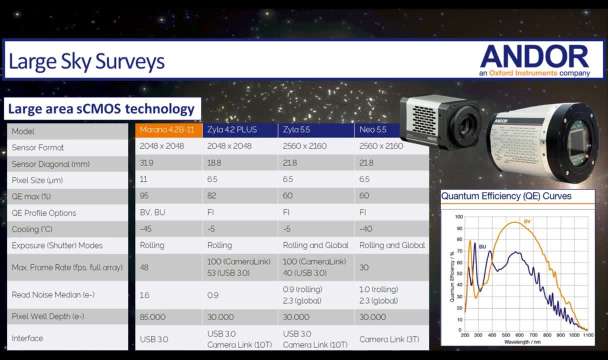 there are also two different sensor options. it comes with a rolling shutter and it offers at full, at full frame, a frame rate of about 48 frames per second and still has a low read noise. and then, if you can also compare that to the xyla 4.2 or xyla 5.5, those are front illuminated sdmos cameras. 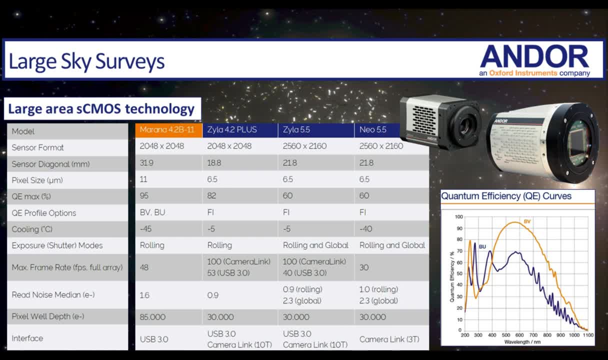 and the good thing, for example, is that they also offer the camera link connectivity that makes sure you can acquire images with about 100 frames per second, and they also have exceptional low read noise of about 0.9 electrons. and then we also have the neo 5.5. this was the camera that emiliano was using for 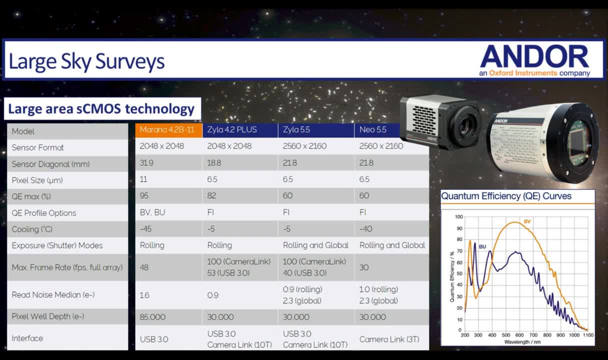 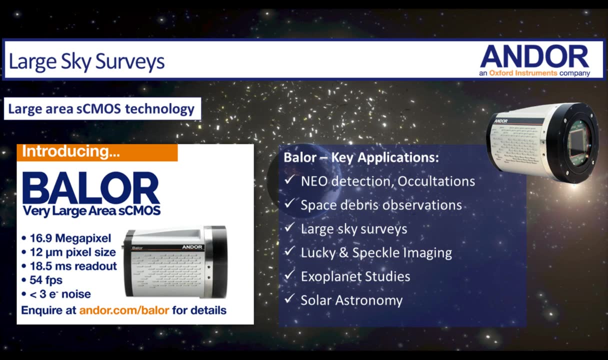 his observation and he also mentioned that in his presentation. so this is a front illuminated sdmos camera. it's cooled a bit further than the xyla and it also offers a true global shutter, which is key for several applications. and then, last but not least, i would like to highlight our newest. 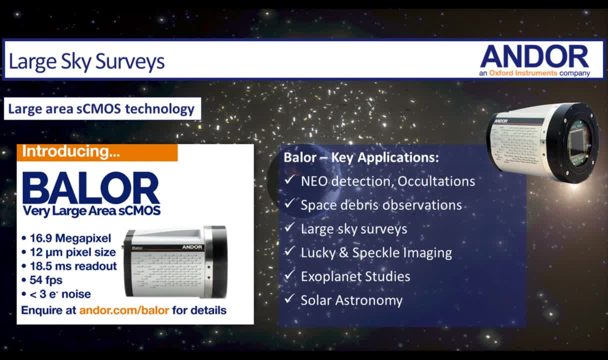 camera development. so that just has been launched and it's called the xyla 4.2 camera, which is a launched about a few weeks ago. this is called the balor. this is a 4k by 4k sdmos device. it has a 16.9. 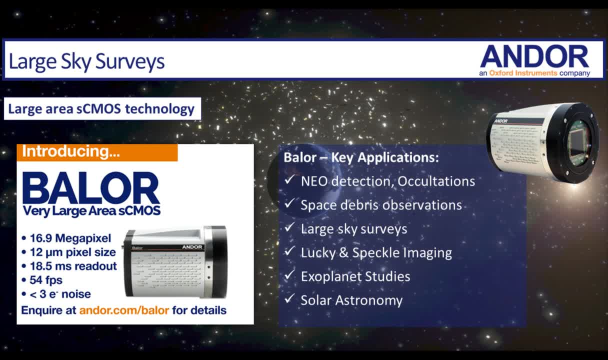 megapixel sensor with a 12 microns pixel size and you can really read out really fast. this is offers a 18.5 milliseconds readout so you can achieve image. you can do imaging with the full frame of 54 frames per second and you can still have. 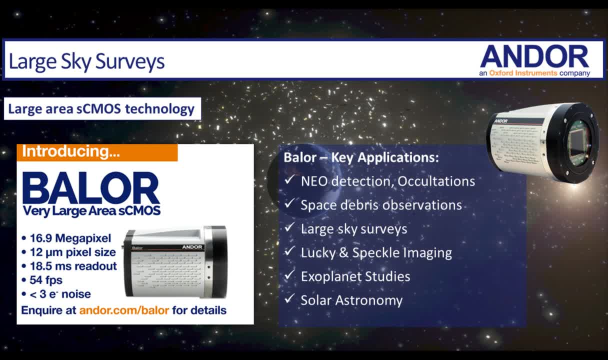 low read noise of less than three electrons so degree. the key applications for this camera are near objects observations, occultation, face degree observation or large sky surveyed- because, like i said, it's a 4k by 4k device, also great for lucky and speckle imaging- or exoplanet studies. 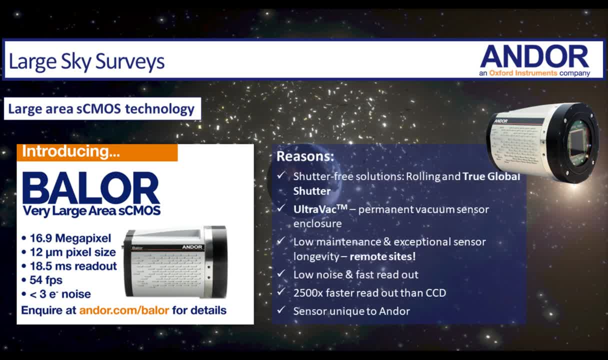 and even solar astronomy. so why are you? why is this camera specifically for action photography? why is this camera especially for action photography? why is this camera specifically clothes as well is this camera suitable for these applications? so one of the reasons is that also, like i mentioned before, that this camera is a has a shutter free solution, so we have electronic shutters. 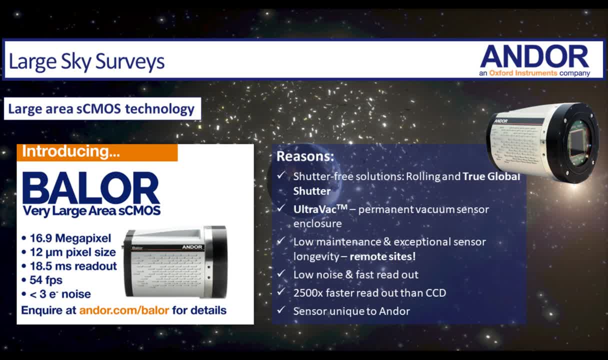 no mechanical. it offers rolling and true global shutter, and especially true global shutter is really important for applications like solar astronomy or orbital debris observations. then the sensor is in a permanent vacuum enclosure and this really makes sure that the camera is a low maintenance solution and also offers an exceptional sensor longevity, because 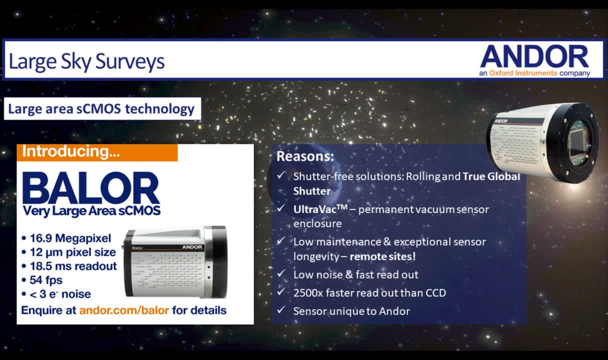 of that. this, in turn, is great if you observe with that camera from remote observing sites, which is very often the case in astronomy- because, yeah, it's really low maintenance and you don't have to touch it, you don't have to do vacuum repump, nothing, you don't have to worry about the shutter. 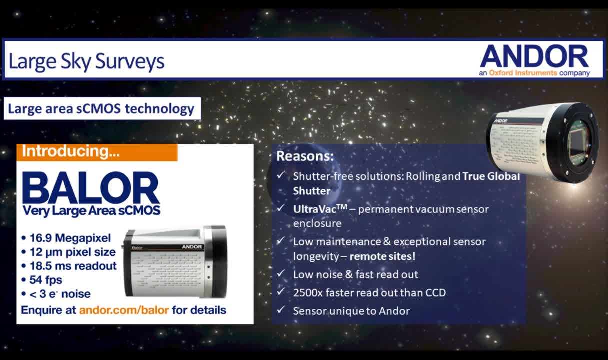 then another good thing is that you have the fast readout but also the low noise level, and that is very different if you compare that to ccd solutions. so if you, for example, take an image you expose 10 seconds with a ccd of similar size, then you would read out in 45 seconds, whereas with the baller. 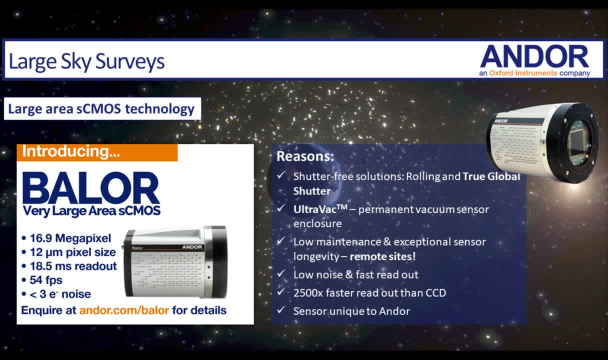 10 second exposure, you would read out in 18.5 milliseconds. so this is really about 2500 times faster than the same with the ccd. and another thing i would like to highlight is that the sensor of the power is unique to under, so it's not a two pixel sensor or whatever that we use. 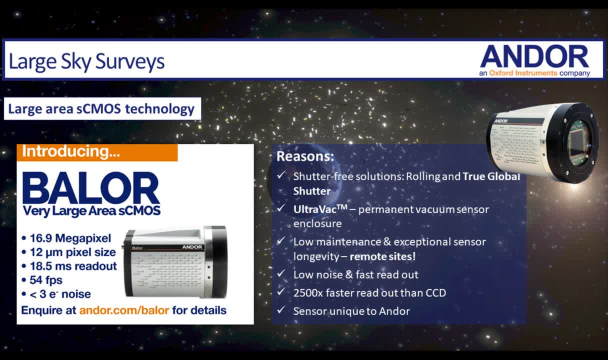 for example, for a mirana camera. it is unique to andorran and just to give you some examples. so the first cameras are used at nasa, jpl or the dickie solar telescope and even in china. so those are several groups that already work with the follower. 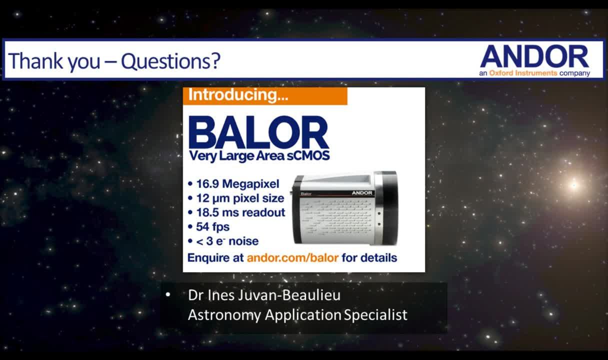 so, yeah, thank you for that. um, please let us know if you have any questions and i will give back to christy. thank you, inez, and thank you, miliano, for your informative presentations. we will now start the live q, a portion of our webinar now to our audience, if you have any. 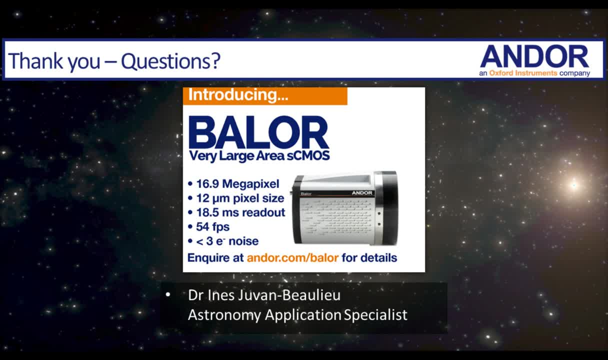 questions you'd like to ask. please do so now. just click on that ask a question box located on the far left of your screen, and we will answer as many of your questions as we have time for it. all right, let's get started. our first question, and you know let's. 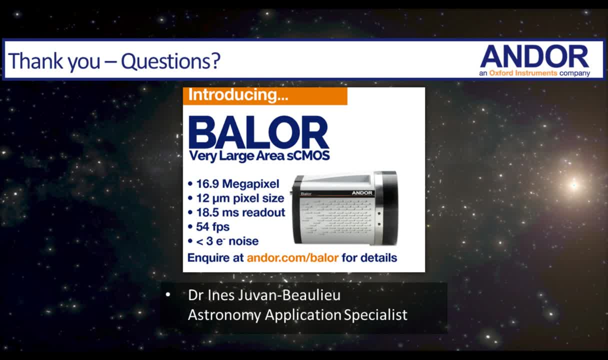 start with you, what differentiates the balor from the other large area as CMOS cameras on the market? Thank You, Christy. so that's a very good question and I just recently did some research on the internet and compared to the balor with different large area cameras on the market and I have to say that I think 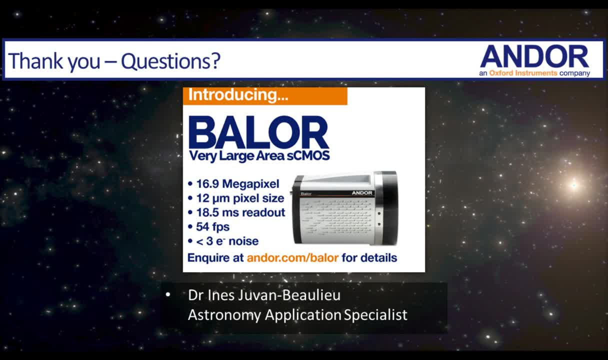 that the balor is the only camera- only a CMOS camera- on the market that has the true global shutter and, as I mentioned that on my slides earlier, that is really key for several applications like, for example, solar astronomy or orbital Libra observation, so that's definitely something that the customer should keep. 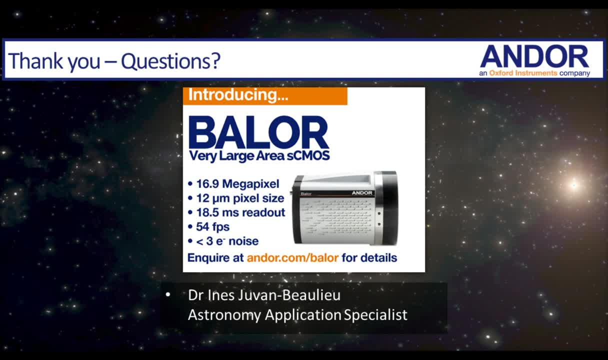 in mind if their application requires the true global shutter mode. and another thing is that I would like to highlight again that the balor sensor is in a unique vacuum enclosure, so that really makes sure that the sensor is protected and offers performance longevity over long time. so I think 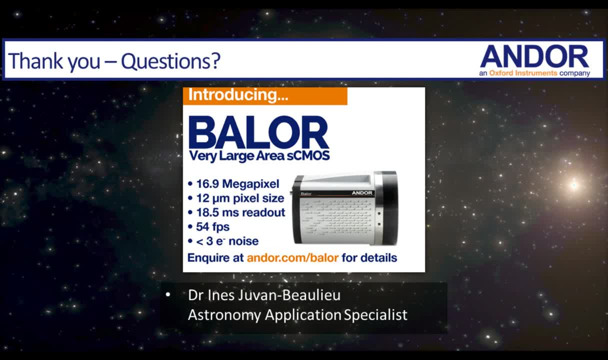 those are the main points. they be also something that the balor has three different gain options, so I think that's also something that I did not see with other in large area👟 CMOS cameras on the the margin. Thanks, Ines. Now, Emiliano, let's jump over to you. What are 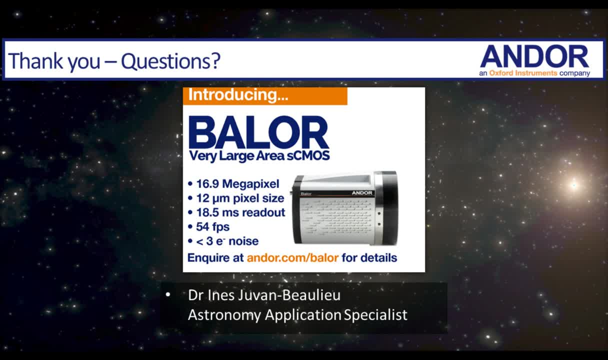 limitations for the LEO observations. Oh thanks, Christy. yeah, good question. Actually, there are several parameters that contribute to the limitation on the LEO observation. It depends a lot on what we want to observe. So in the space debris world, especially for LEO observation, we are looking for small. 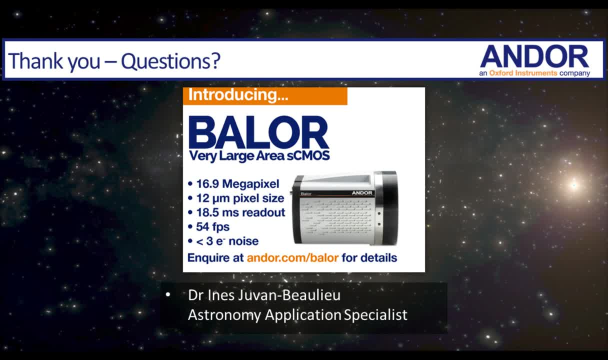 objects. Looking for small objects usually requires a big aperture telescope. Then the problem is that we don't have a big aperture telescope. So the problem is that we don't have a big aperture telescope, Then the problem is that, like, okay, big aperture telescope usually. 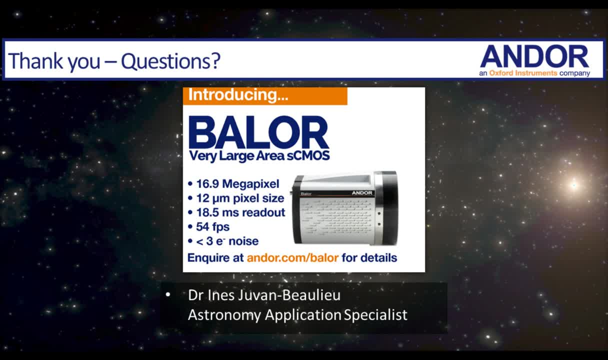 correspond to a relatively long focal length, So that means that the field of view is small. Then, if you want to, the discovery becomes quite difficult. then what we can do is even if we are looking forward this kind of object. the problem is that smaller objects need a longer exposure time, even with the bigger field of view. 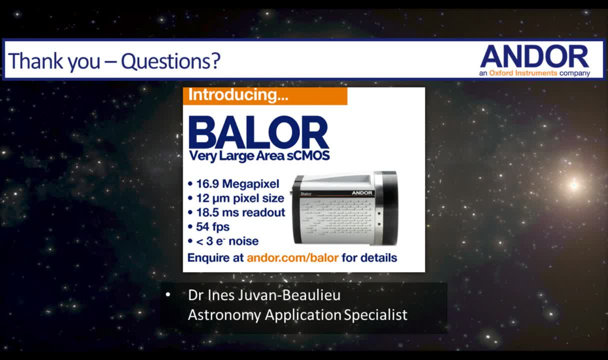 then if we want to use a longer exposure time as an example, we'll have a problem that following an object that is moving fast with longer exposure time in a small field of view either ends up in long star streaks in the image and that our software is not able to process. 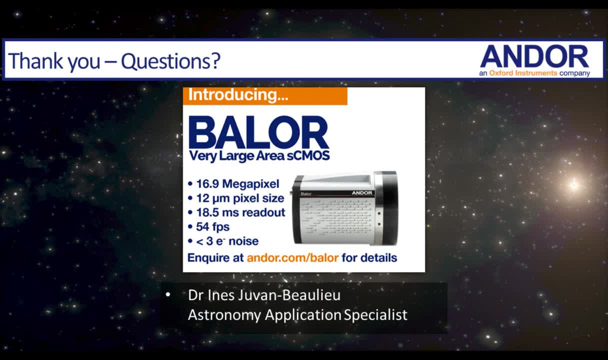 because maybe they are not all included in the image. and secondly, is the number of stars that you see in the image. so, moving the telescope faster, you will have only the brightest star in the image. but then if you have only the brightest star and you have a small field of view, 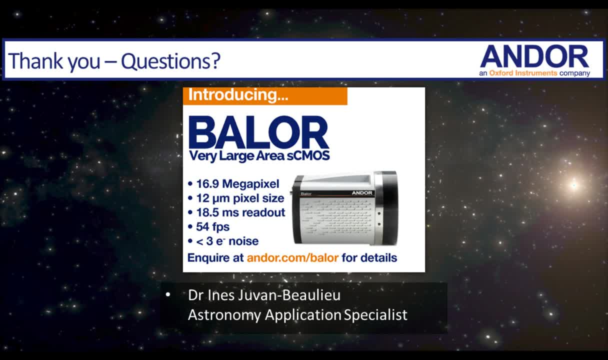 maybe you don't have enough star in general to perform an astrometric data reduction. this is one of the limitation. the second, another one that they would add is the time tagging of the measurement. so if you want to do or be determination, it's important that we 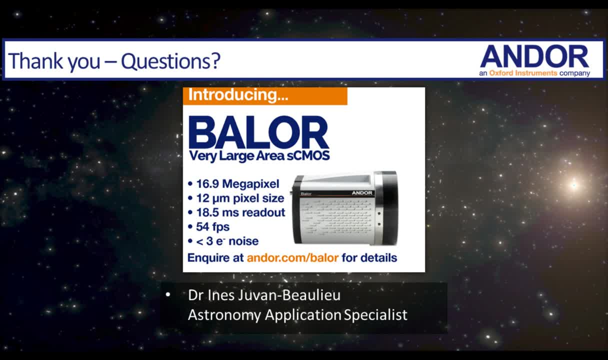 are able to time tag precisely our picture and for CCD observation it works. I would say, if we use a longer exposure time, that are not in agreement with what we I have just said. so because the uncertainty is given by the mechanical shutter. using a mechanical shutter usually takes 50 milliseconds to open. 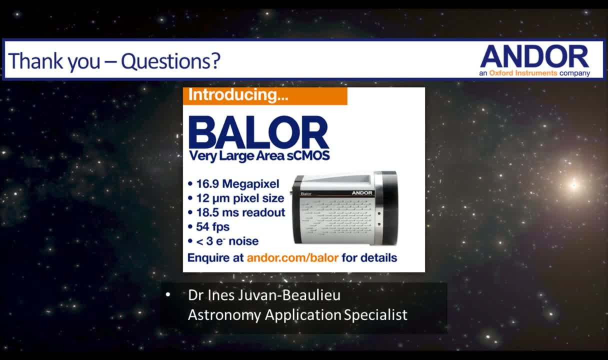 other 50 milliseconds to close, then you have an uncertainty of 50 millisecond. when, let's say, when time taking our measurement for a Leo 50 millisecond, we are talking about how much 350 meter of insert uncertainty, then this is another limitation we should. 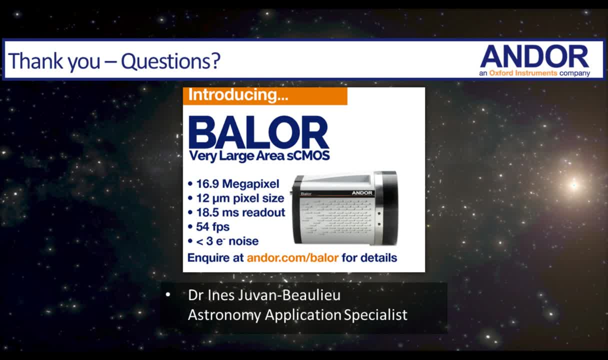 stay on the millisecond level, accuracy, and for these I think is easier to use an electronical shutter. now, Emiliano, while we're talking about your telescope, can you tell us what the smallest object you can observe is? okay, oh, also here a nice question, but there are some parameters that one should consider as an example. we let's 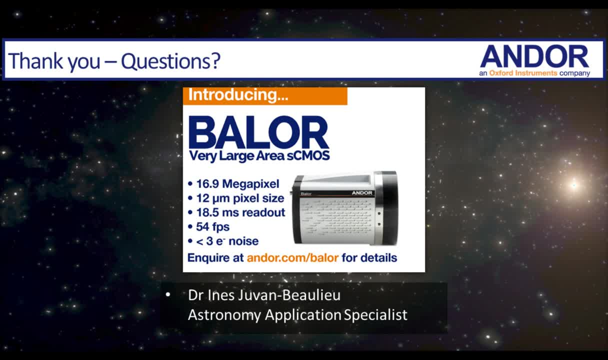 consider: we have different telescope here from 20 centimeter in aperture till one meter size. aperture depend on the, of course, on the quantum efficiency, depend a lot on the sky background and, let's say, the aperture of the telescope. for the 20 centimeter telescope, doing some assumptions on the hyperbola reflectivity of the object, I would say 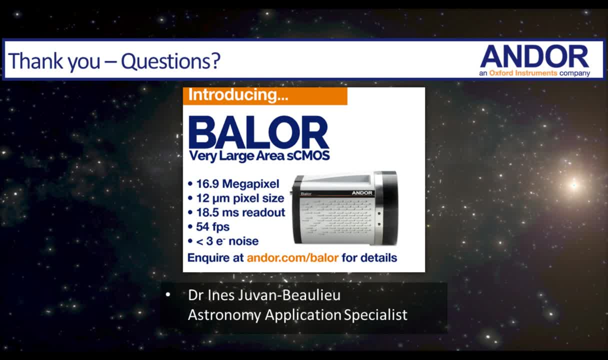 with 8 seconds of exposure we are able to get meter size object if we didn't move to the one meter telescope other- sorry, I was forgot. other parameter that influenced the small size of object that one can see is the exposure time and the How much time we are integrating and the distance of the object. So for the 20 centimeter telescope, for the 1 meter size that I was telling you is at 36,000 kilometers at the geostationary altitude with 8 seconds of exposure. 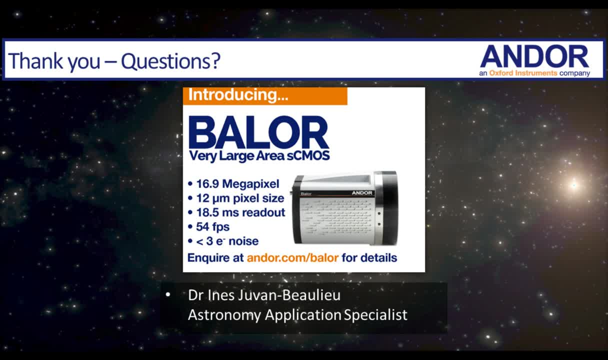 With the 1 meter telescope we are able to detect a CubeSat of 10 by 10 by 10 centimeter at 700 kilometers, with half of a second of exposure And with 8, 10 seconds of exposure we are able to detect 20, 30 centimeter at the geostationary altitude. 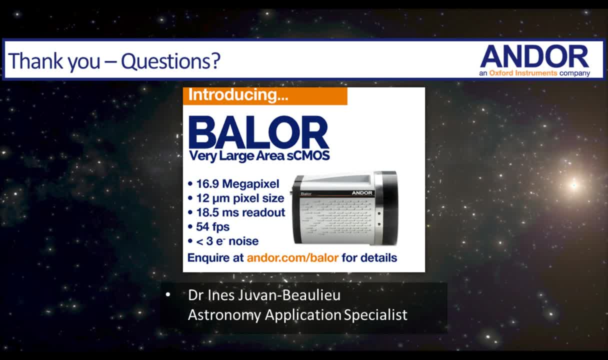 Thank you, Emilio. Thank you Emiliano. Now, Ines, let's come over to you. What is the timing accuracy of the BALOR? Okay, yeah, that's also related to that question, to that topic. So the BALOR offers IRIC-B GPS timestamp connection And that means it allows imaging with a GPS timestamp of a resolution of 10 nanoseconds, So that really allows you to think across multiple instruments and multiple objects. 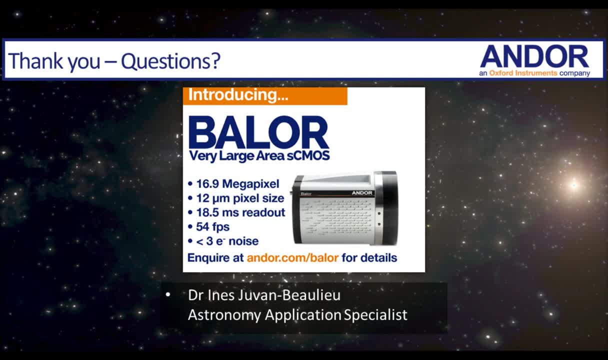 So that's really a great feature. And, yeah, the resolution is 10 nanoseconds. Thank you, And now our next question: what is the difference between rolling and global shutter? Yeah, I guess I should have mentioned that earlier. I've been talking about that quite a lot, But yeah, the difference is that if you have a rolling electronic shutter, that means that I mean the pixels in each row are all exposed. 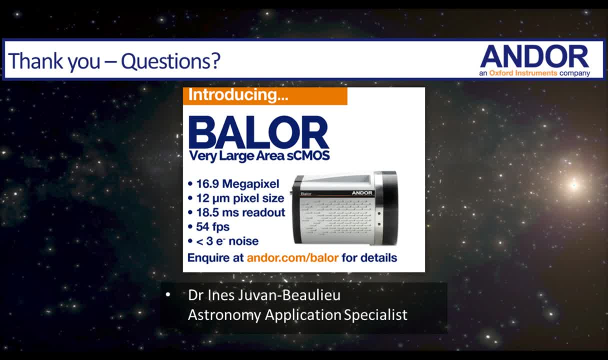 Basically, the images are exposed for the same amount of time, so they have the same exposure time, But the start and the end of this exposure time is slightly different with each row And in comparison to global shutter. so there you really take a snapshot of your image And that means that really every pixel is exposed for the same amount of time and at the same amount of time. So that's the slight difference. 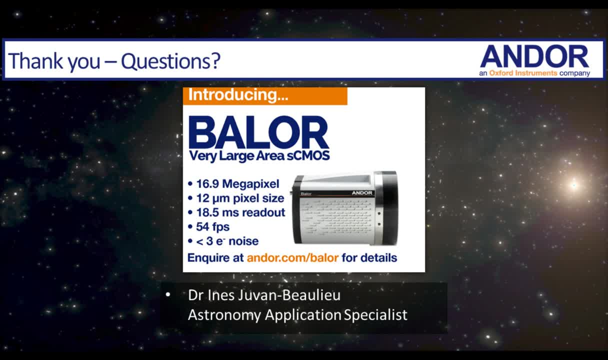 But this can be crucial for applications that really require this time, a precise time correlation. Thank you, Inez. Now looks like we have time for one more question, but I would like to quickly remind our audience that any questions we did not have time to answer today and those that are 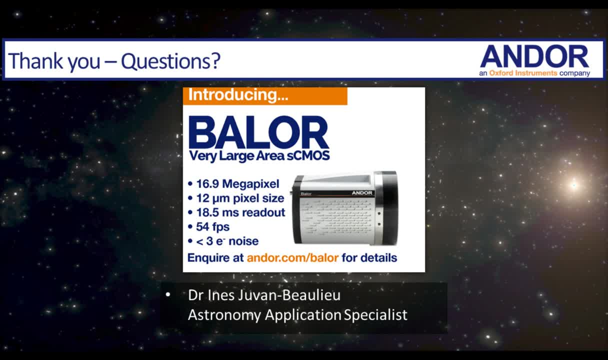 submitted during the on-demand period. they will be addressed by our speakers via the contact information you provided at the time of registration. And, Emiliano, let's end with this question for you: What strategy do you use to observe? Okay, let's talk about space debris One. we have to make a distinction, Even if at the end, 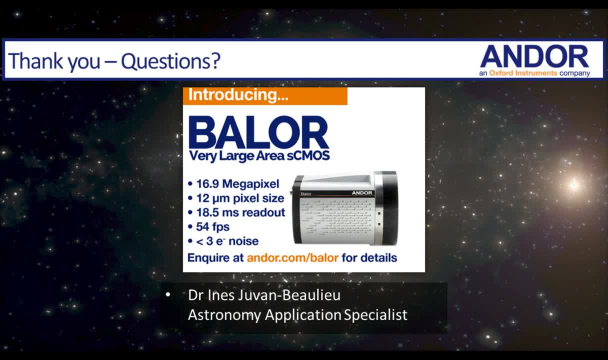 the images will look like similar. we have to make a distinction. what we want to do? Do we want to distinguish? Do we want to discover space debris Or do we want to improve the accuracy of the orbit of an object that we already know? So in the first case, we are talking about survey In a survey. 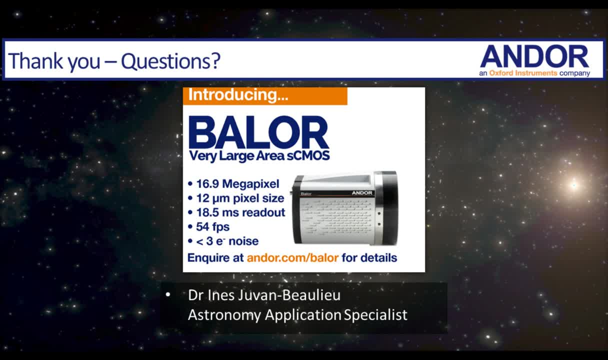 usually we point the telescope in the sky. The region of the sky usually is not completely random, but usually you look to a particular region that should be populated by debris And populated by a certain kind of debris, As an example, if you want to do a geostationary survey. 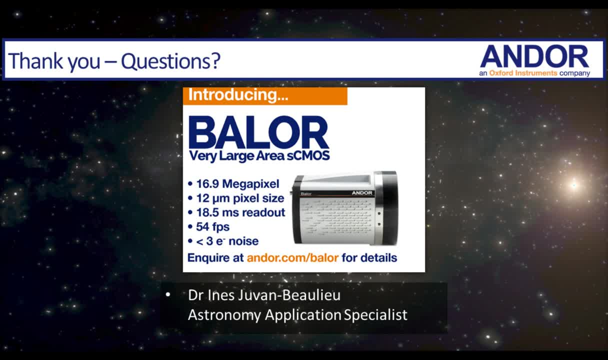